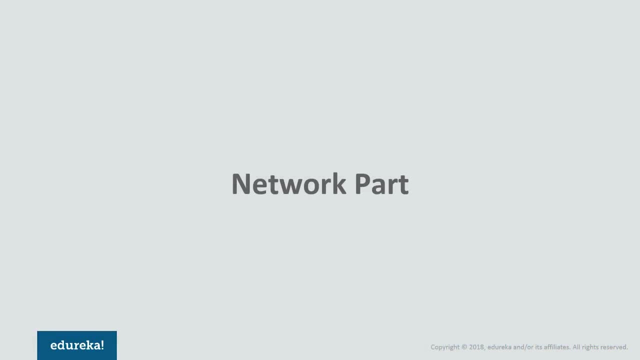 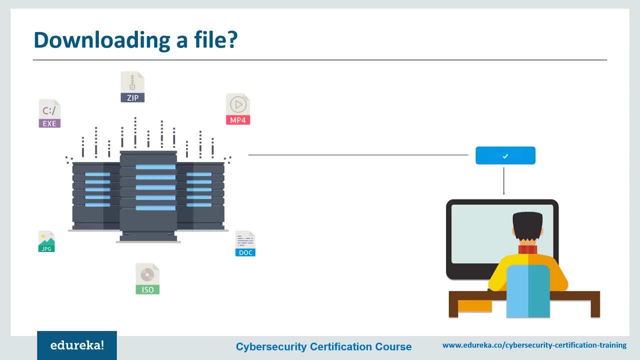 Okay, So first we're going through the network part and I'm going to teach you all how a network actually works. Okay, so I think it's right to assume all of you watching this video have downloaded some sort of file in the past, whether it be a movie, a TV show, some software. 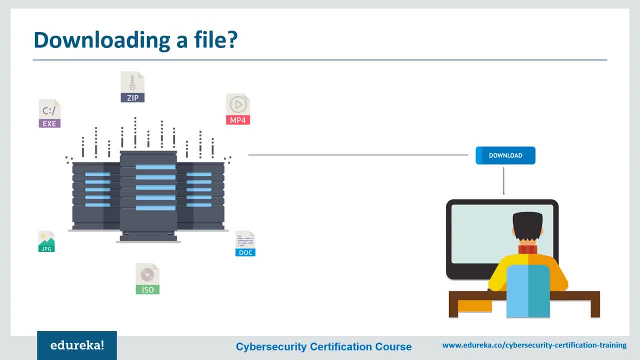 or music. you have downloaded something off the internet, but most of you don't really know how the whole process works. Now let me take a moment to explain the whole thing. So first of all, when you click that juicy download button, your whole file doesn't really get sent to you all at once. 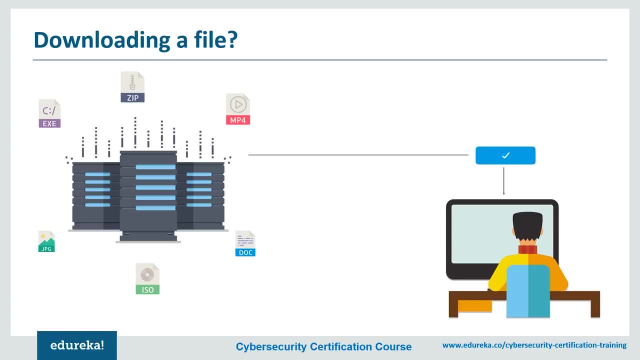 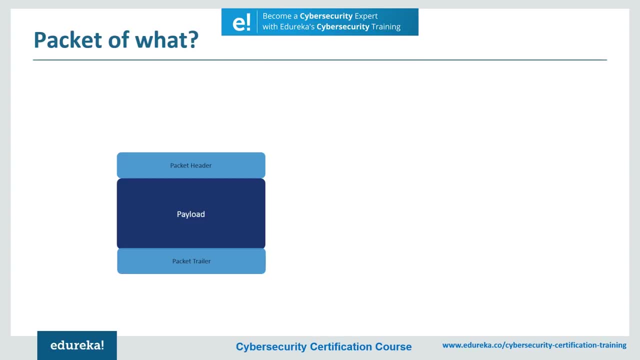 rather it is broken down into tiny units called packets, which are then transmitted over a network to your computer. Now the way how atoms make enormous objects together. data packets come together to form one big file. They can be considered the atom of a network, and like an atom, a data packet 2 has a pretty complex structure. 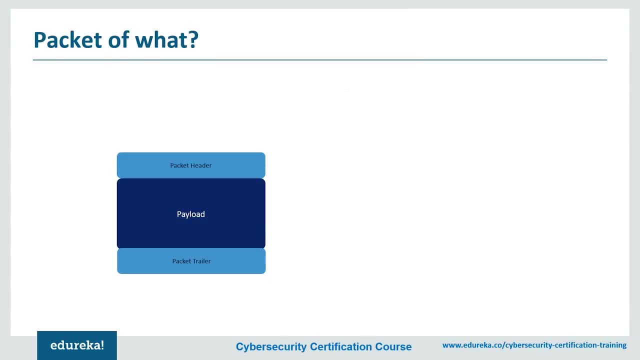 which can be broken down into three significant parts, namely: The packet header, which generally contains critical information about where the packet is coming from and where it is headed. the payload, which is basically the data contained by the packet. and the packet trailer, which is dust data to signify the end of a packet. now 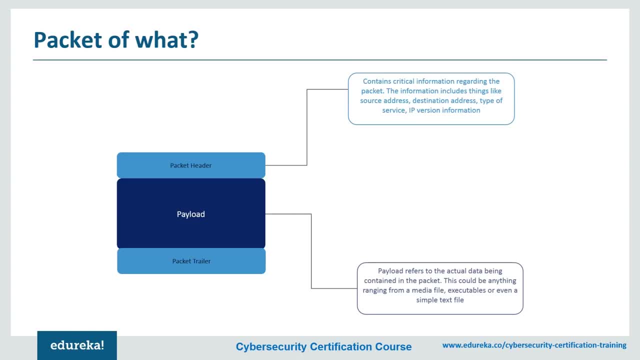 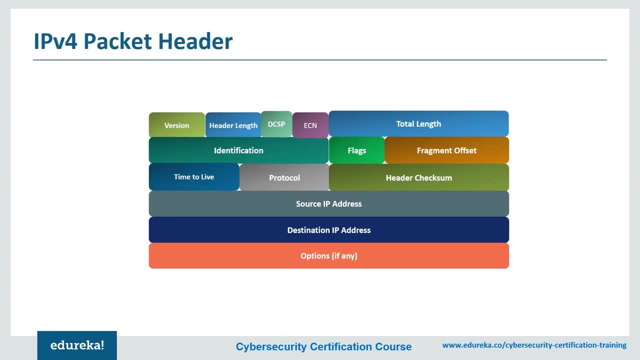 out of the three, the packet header is the most important to understand when understanding the structure of a network, So let's have a deeper look at it. Okay, Now, what do you see on your screen at this moment is an IPv4 packet header. a little bit on IPv4 before we continue. 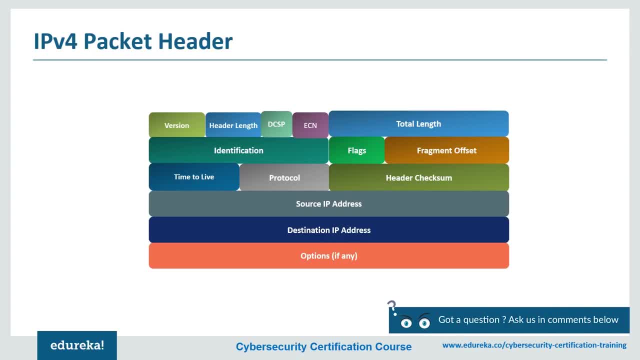 is that IPv4 is the fourth version of the internet and it is also the most widely used digital communication protocol. There's also IPv6, but it hasn't really been implemented widely. and about IPv5. Well, let's say it's what Microsoft it with Windows 9.. 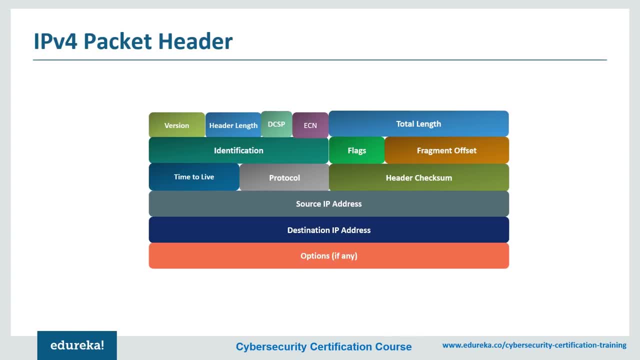 It doesn't exist. Now It's pretty evident from what we look at that the IP header indeed is a complex structure with numerous parts. the IPv4 packet header consists of 20 bytes of data, and option part also exists within the header that allows for the optional bytes to be added. 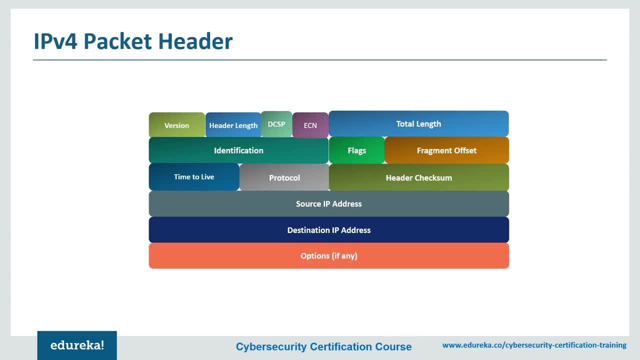 But this is not normally used, with the occasional exception of something called a router alert. Now let's take a moment to discuss all the header files briefly. So first fall, we have the version part. Now this is always set to four in the current IP version. 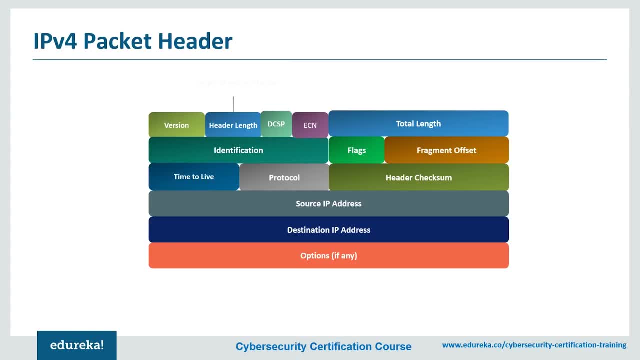 and it shows the version of the protocol that we are following. Next is the header length, or the IP header length, and it's a number of 32-bit words forming the header, which is usually five. Next is the DC SP field, which is for differentiated service code point. 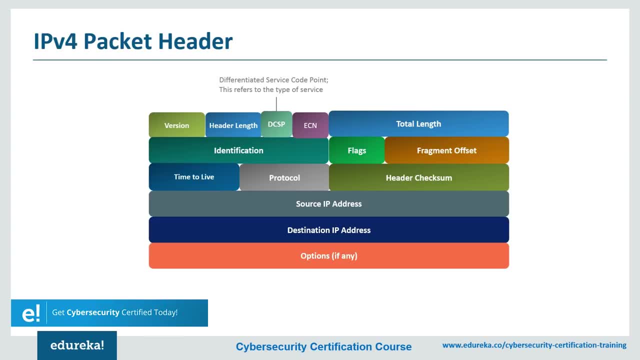 It is a 6-bit field, sometimes set to zero, but can indicate a particular treatment, sometimes reflecting the quality of service needs of an applicant to the network, and the DC SP informs a router how to queue packets while they are waiting to be forwarded. Next is the ECN field, which stands: 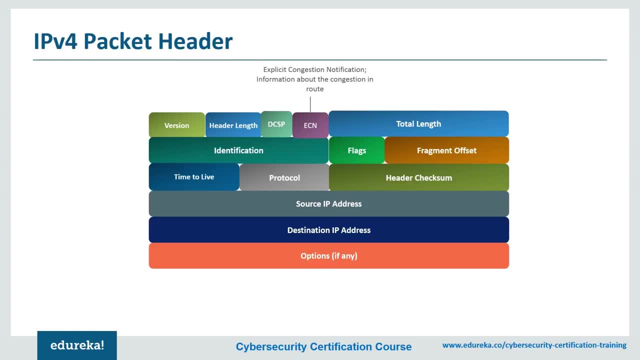 for explicit congestion notification and it tells us about the congestion in the network route. Next is this total length, which is the size of the datagram, and this is in bytes, and this is the combined length of the header and the data together. Next comes the identification field. 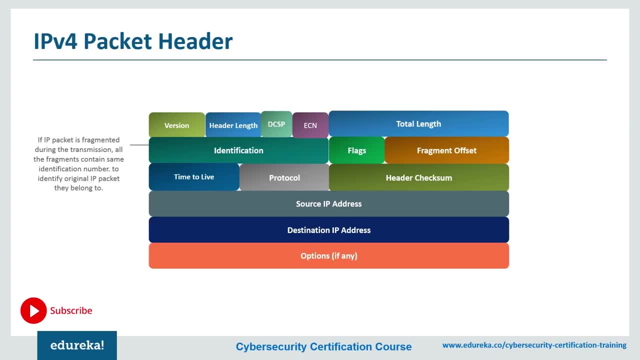 Now the identification field is a 16-bit number which, together with the source address, uniquely identifies a packet that is used during reassembly of a fragmented datagram. Next is the flag spot. Now there are sequence of three flags. One of the four bits is unused. 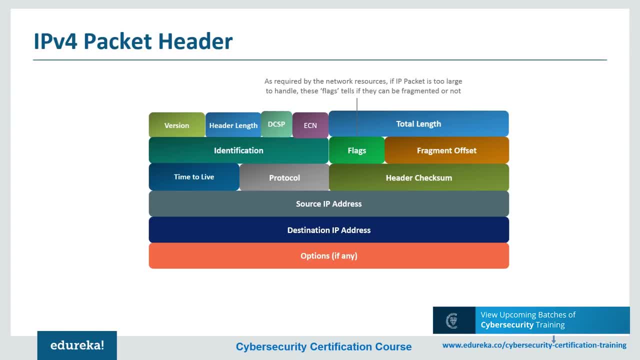 and used to control whether the routers are allowed to fragmented packet and to indicate the parts of a packet to the receiver. Next is the fragmentation offset and this is the byte count from the start of the original send packet sent by any router which performs IP router fragmentation. 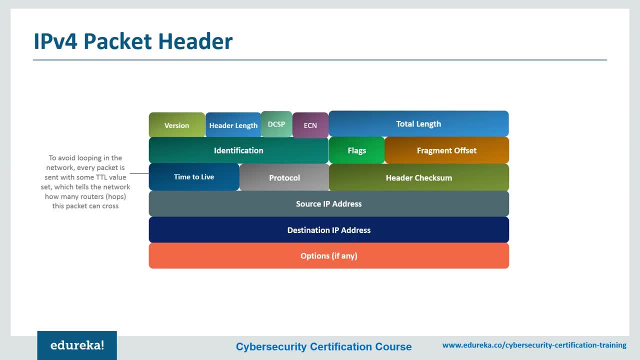 Next is time to live. Now, time to live is the number of hops or links which the packet may be routed over or decremented by most routers used to prevent accidental routing loops. It's a very important aspect of every packet. Next comes the protocol. 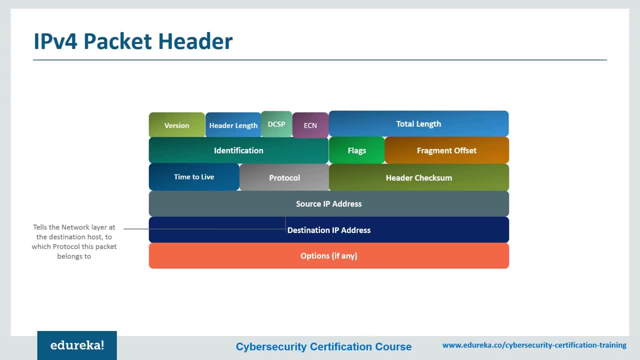 Now the protocol is a service access point, or SAP, which indicates the type of transport packet being used and carried. For example, if it's one it's ICMP, If it's two it's IGMP, If it's six it's TCP and if it's 17,. 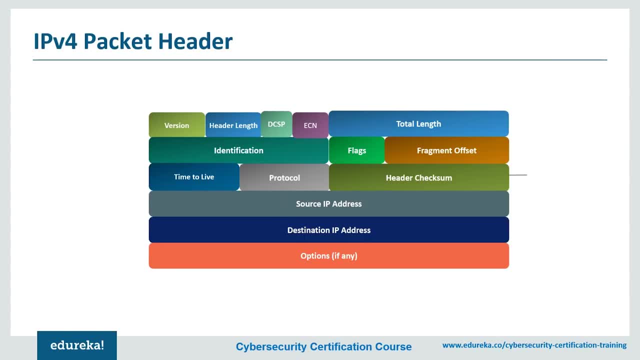 it means it's following the UDP protocol. Next is the header checksum. Now a once complement checksum is inserted by the sender and updated whenever the packet header is modified by a router, and it is used to detect processing errors introduced into the packet inside the router or bridge. 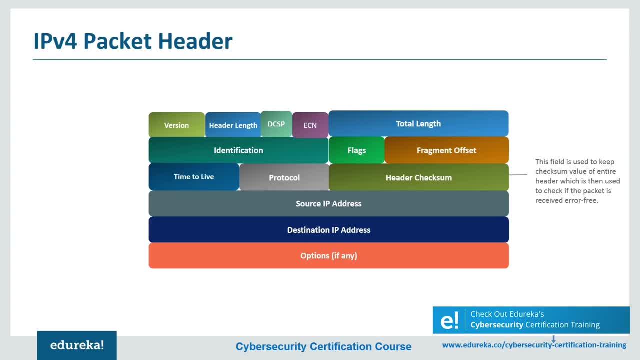 where the packet is not protected by a link layer. cyclic redundancy check. Now packets with an invalid checksum are discarded by all nodes in an IP network. The checksum can be thought of something like a barcode. if the barcode gives you wrong information, You just discard that packet. now. 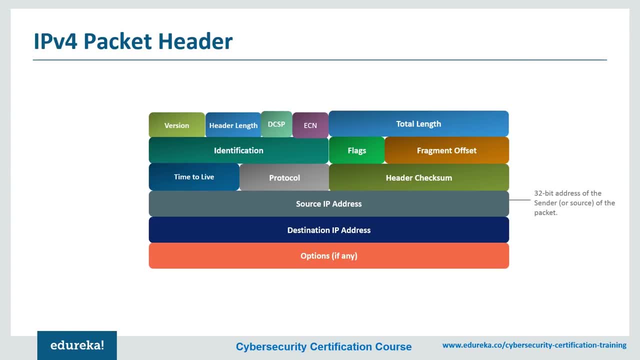 as you guys can see, the next field is a source IP address, and it is the IP address of the original sender of the packet, and next is the destination address, which is the destination field of the packet. and then we spoke about the options field. Now, it is not normally used. 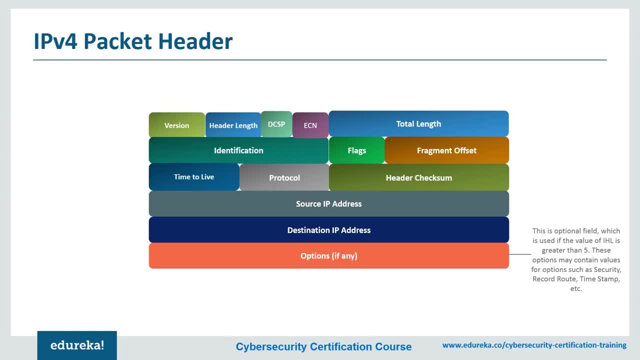 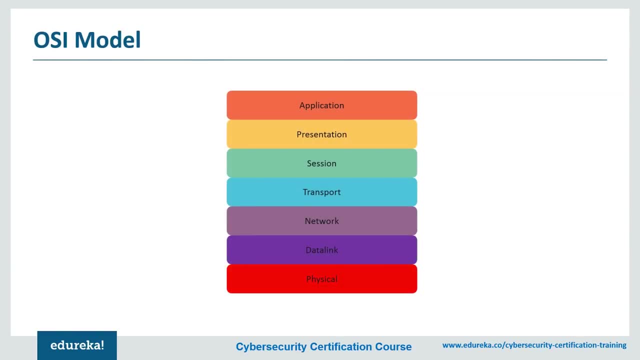 but when used, the IP header length will be greater than 5 32-bit words to indicate that the size of the option field has been included. Now the internet protocol has been there for a long time and there has been a couple of models that have really given the protocol a structure. 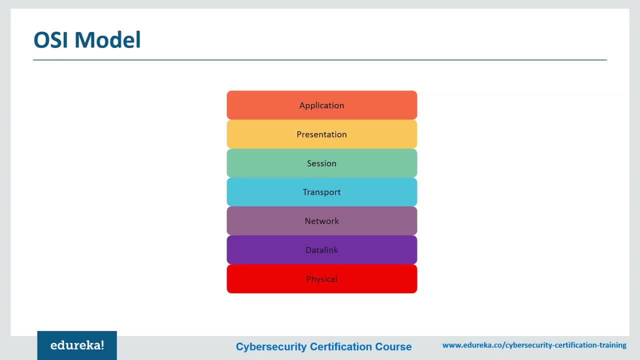 The first model is called the OSI model and the second TCP IP. now, both these protocols have a layered stack architecture, with each layer having very similar functionalities. First of all, let's have a look at the OSI model now. communications between machine is hard. many, many details. 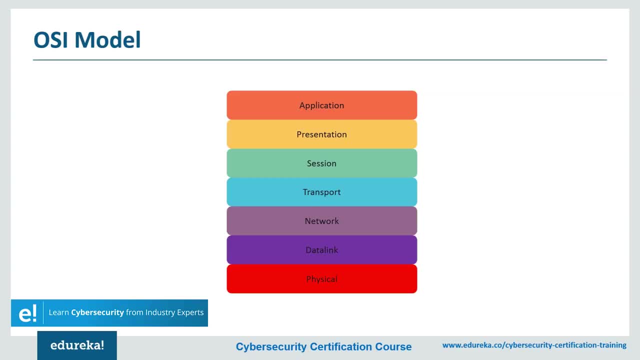 and considerations are important in order to relay some information from point A to point B, and therefore every system is left on its own and has a tendency to be very different. The OSI layer model was made as an effort to divide the process of communication into a number of steps. 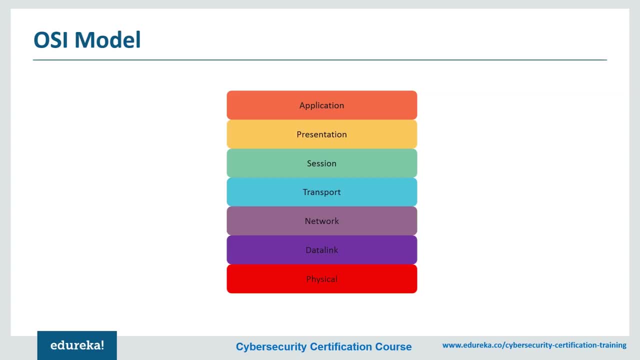 So every step could tackle some of the needed functions of the transmission separately. Now let me use a very strange analogy to explain all the functions of each of the layers in the OSI model. So suppose you want to send a number of objects, Let's say a group of vases, to a friend of yours. 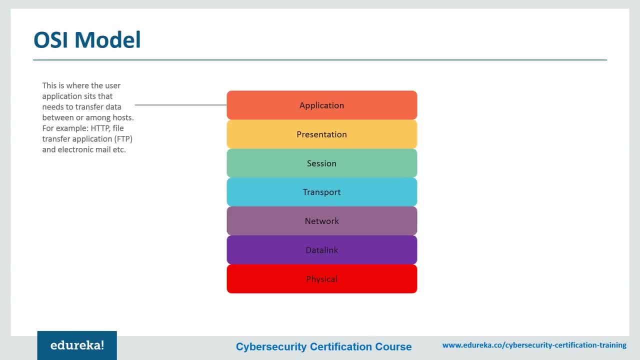 that lives on the other side of the world. He needs the said vases in order to put on some plants on a display. now, you and your friend represent layer 7,, which is the application layer, which makes the final use of the sent object. 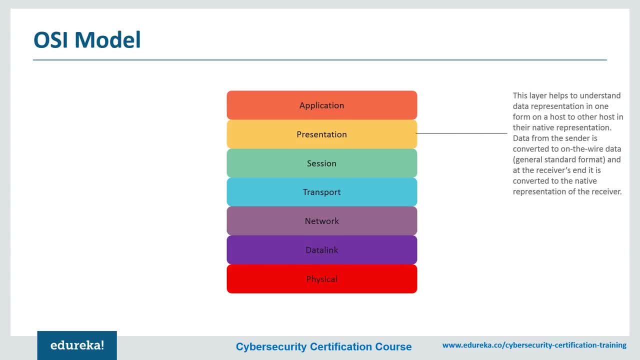 Now you give this ways to another person. Let's call him a professional packer. He takes your vases, puts it in several boxes, fills them with wrapping in order to prevent it from breaking and closes the boxes completely. this professional packer represents layer 6,. 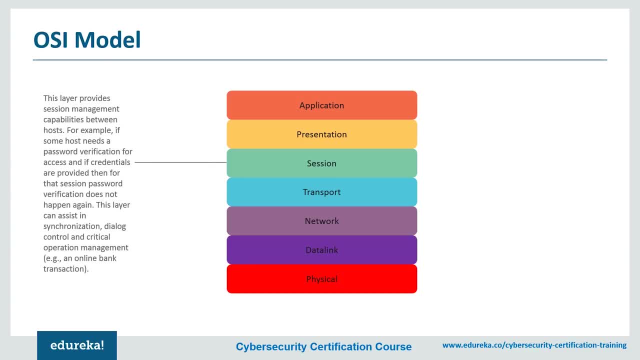 which is the presentation layer. Now this professional packer takes all the boxes, gives them to a guy and arranger. now He doesn't know what is inside the boxes, but he knows they all go to the same friend of yours, So he labels them appropriately. so far. 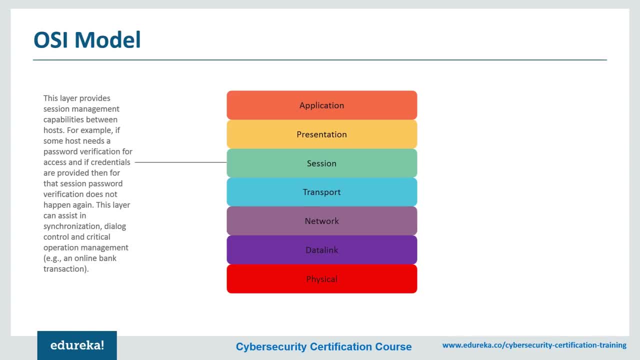 He represents layer 5 and that is the session layer. Now the arranger takes all the boxes down to an office who handles clients and Dawson's of other buildings. They keep in touch with hundreds of other agencies at the same time. They do not actually send the boxes. 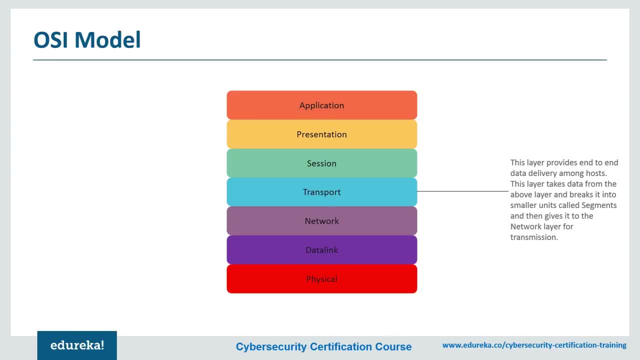 but they track them and know when a box for an order is missing, and so these guys are layer 4, which is also called the transport layer. Now, one of the guys from the office actually takes all your boxes, along with many others, to a post office. 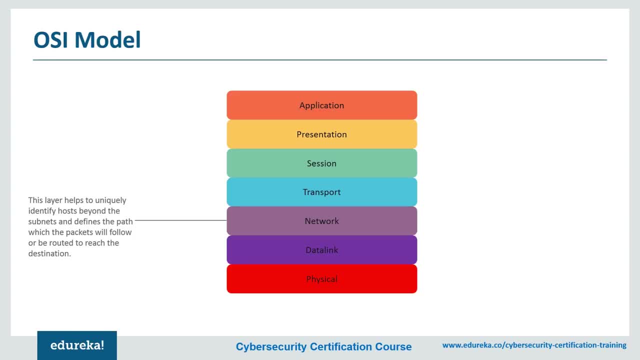 This post office is the third layer. here It is given an address- the one of your friends- and this is the layer 3, that is called the network layer. Now one of the guys from the post office takes all the boxes to a dock and the guys 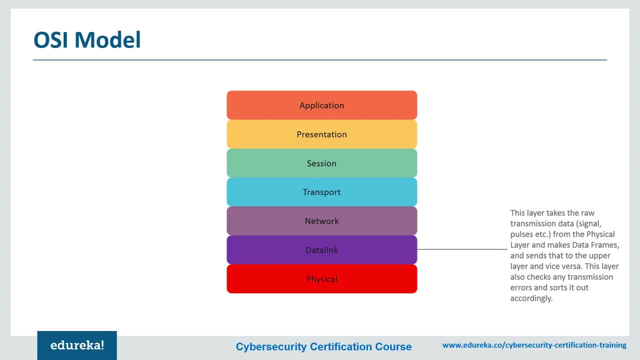 at the dock, pull all the boxes into a container. They know very little about what the boxes contain or where their final destination is. They only care about which other dock is this container headed to. Now this dock is representing layer 2, which is the data link layer, and finally we have the ship. 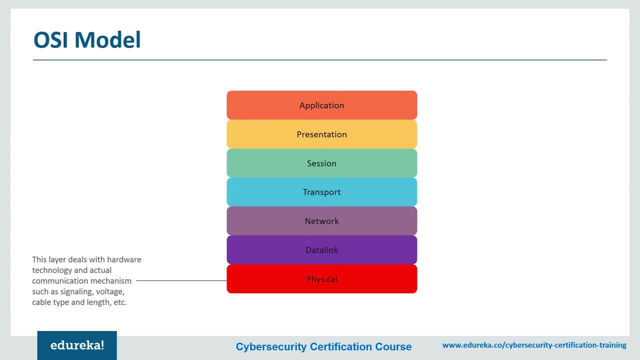 It only knows where it is headed and takes the container with it. It handles the waves, the conditions of the sea, the weather and all the other physical conditions that none of the other layers have to deal with. The ship is layer number one, which is the physical layer. 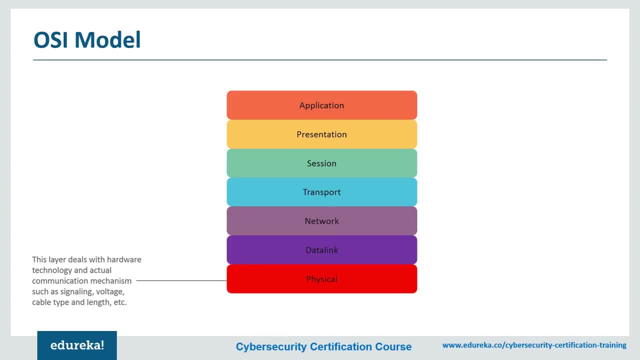 Now, after all this, the ship gets to port, the containers are opened out here. now boxes which are meant for this address stay on the dock and the others are put into other containers and another ship and sent on its own way. Now all the staying boxes are sent to an associated post office. 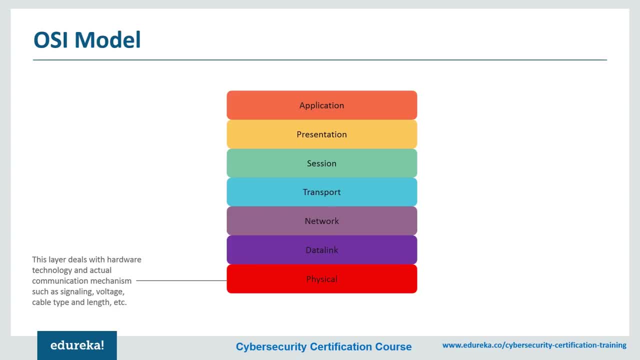 and layer 2 has done its job. Then the post office receives the boxes, maybe realizing some are missing. They call the sending post office to check what happened and once they are sure all the boxes are there, They send it to the big office. and now layer 3. 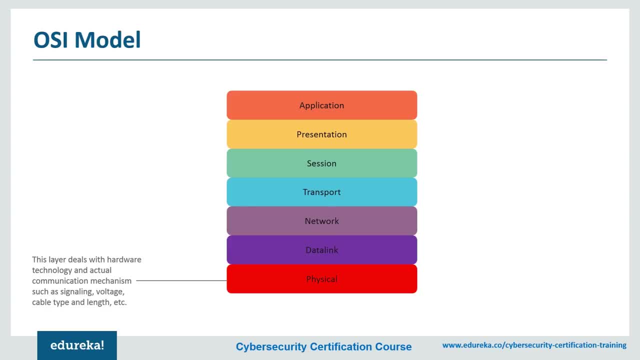 has done its job completely. Then the big office gets the boxes, checks They are all in the correct order and place, fill the relevant tracking data and send them to your friends. Arranger and layer 4 has done its job Completely. Then the Arranger reads the label put by your Arranger. 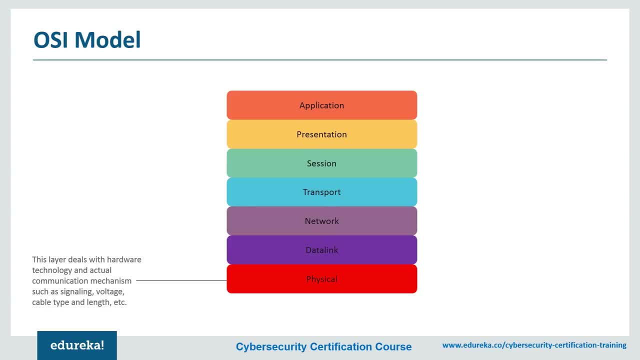 and he makes sure everything is in order. He knows they are for your friend and calls a professional Packer here. Layer 5 has completed its job. Then the professional Packer takes everything from the boxes, checks if everything is intact and if everything is okay. 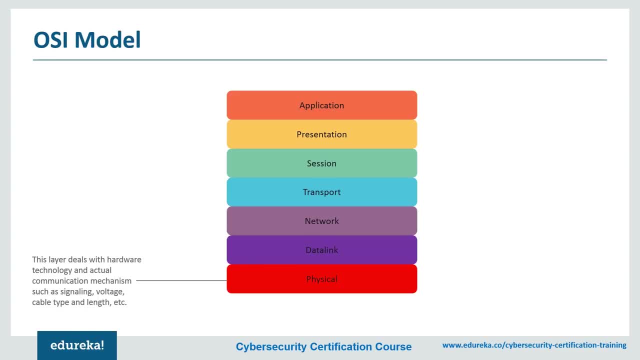 he calls a friend and layer 6 has done his job. And finally, your friends get the vases. happily, unaware of everything that happened on every layer, He sets up the plants on display and is happily continuing with his day. Now, this is how the OSI layer model has actually differentiated. 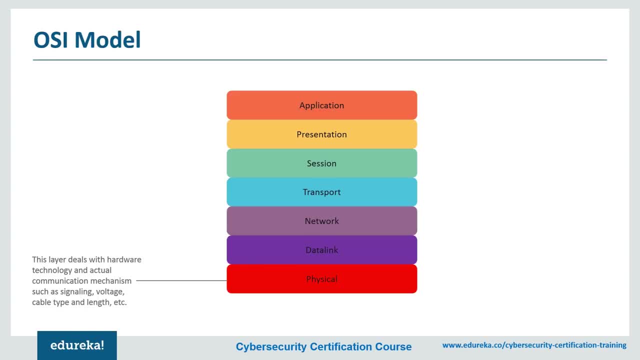 all the different steps that you need for one packet to reach from one computer to another. I hope that analogy helped you all understand how a packet actually travels from one computer to another. Okay, so it's time now that we discussed the TCP IP model. TCP IP. 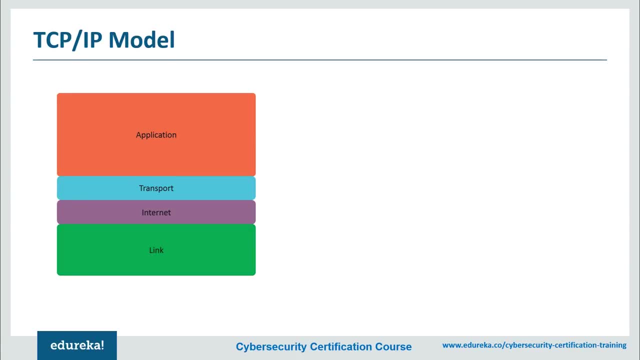 specifies how data is exchanged over the internet by providing end-to-end communication that identifies how it should be broken into packets: addressed, transmitted, routed and received at the destination IP. now, TCP IP requires a little central management and it is designed to make networks reliable with the ability to recover automatically. 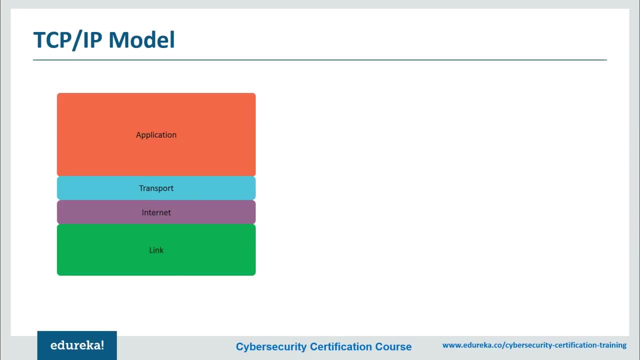 from failure of any device on the network. The advantage of TCP is that it is non-proprietary and, as a result, it is not controlled by any single company. Therefore, the internet protocol suit can be modified very, very easily. It is compatible with all the operating systems. 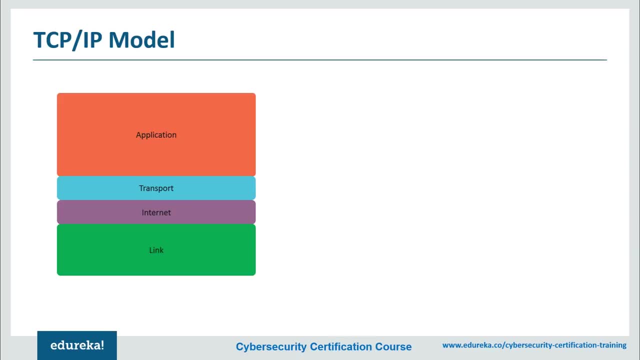 So it can communicate with any other system on the network, and the internet protocol suit is also compatible with all types of computer hardware and network types. Now the TCP IP functionality is divided into four layers, each of which includes a specific protocol. The application layer provides applications. 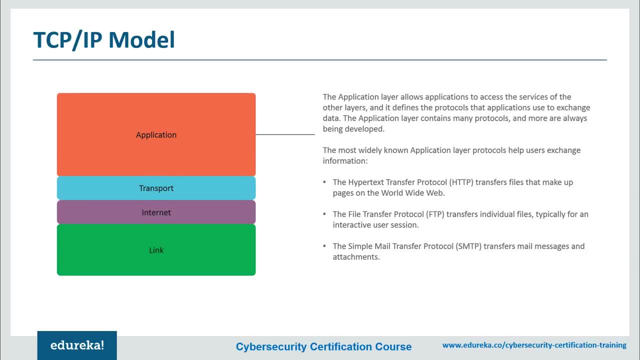 with standardized data exchange. Its protocols include hypertext transfer protocol, which is HTTP, file transfer protocol, which is FTP, post office management protocol, which is POP3, simple mail transfer protocol, SMTP, and simple networking management protocol, which is SNMP. next is the transport layer. 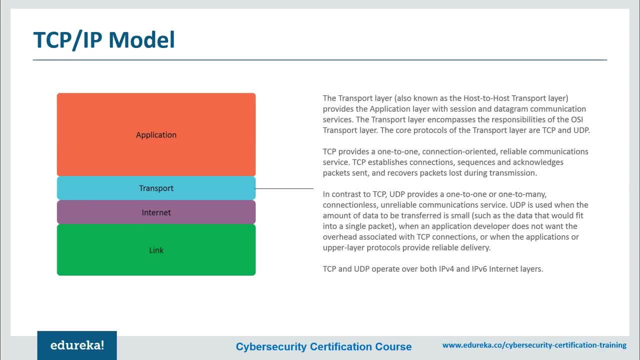 The transport layer is responsible for maintaining end-to-end communication across the network. TCP handles communication between hosts and provides flow control, multiplexing and reliability. The transport protocols include TCP and a user datagram protocol, which is sometimes used instead of TCP for special purposes. 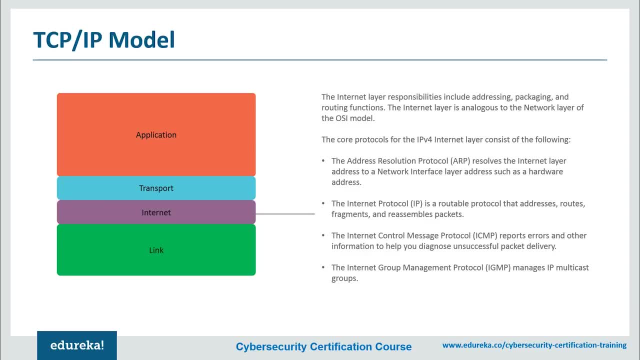 Next we have the network layer. Now the network layer, also called the internet layer, deals with packets and connects independent networks to transport the packets across network boundaries. The network layer protocols are the internet layer, which is the IP protocol, and the internet control message protocol. 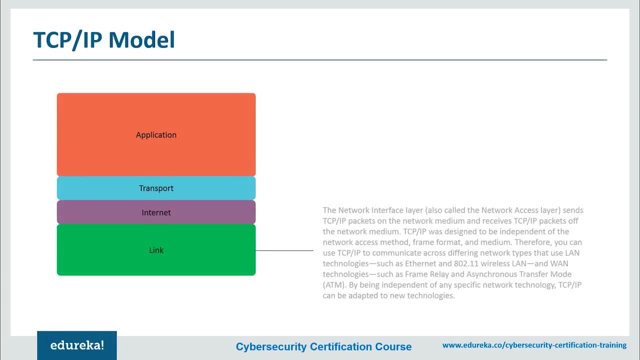 which is also abbreviated as ICMP. last but not least, We have the physical layer now. the physical layer consists of protocols that operate only on a link, that is, the network components that interconnects nodes or hosts in the network. The protocols in this layer include Ethernet. 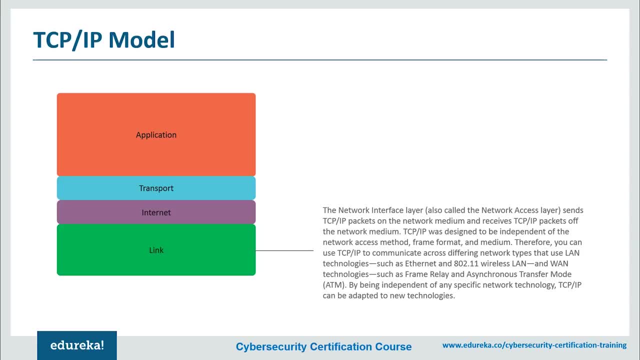 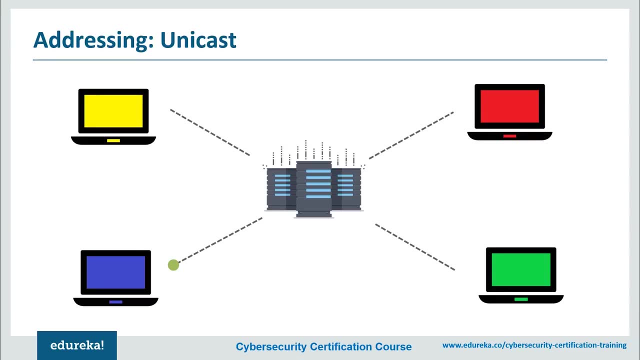 for local area networks and address resolution protocol. So now that we've discussed the models which describe the architecture, Let's move on to the different ways packets can be addressed to other devices. majorly, three main ways of addressing, namely unicast, broadcast and multicast. 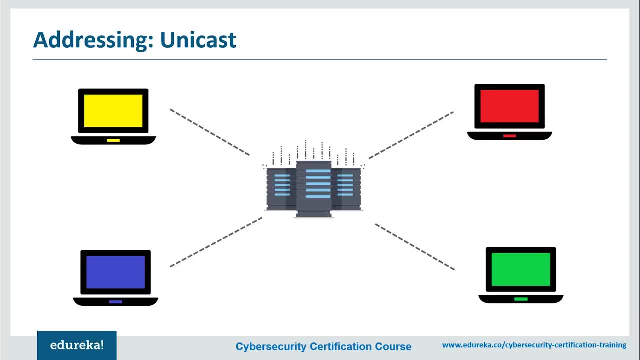 Now, unicast is a term used to describe communication where a piece of information is sent from one point to another. In this case, There is just one sender and one receiver. unicast transmission, in which a packet is sent from a single source to a specified destination, is still the predominant form. 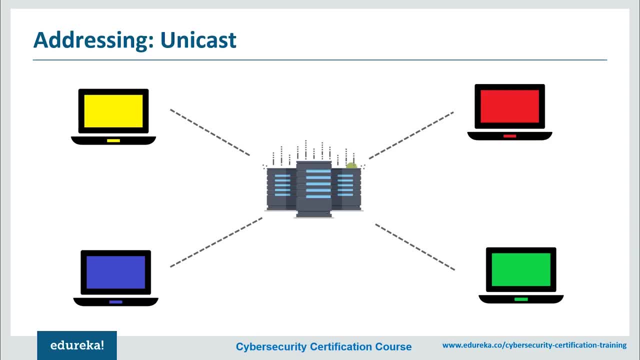 of transmission on local area networks within the internet or local area networks. example: the Ethernet and IP network support the unicast transfer mode and most users are familiar with the standard unicast applications, example: HTTP, SMTP, FTP and telnet, which employ the TCP transfer protocol. The second type of transmission is broadcast, now broadcast. 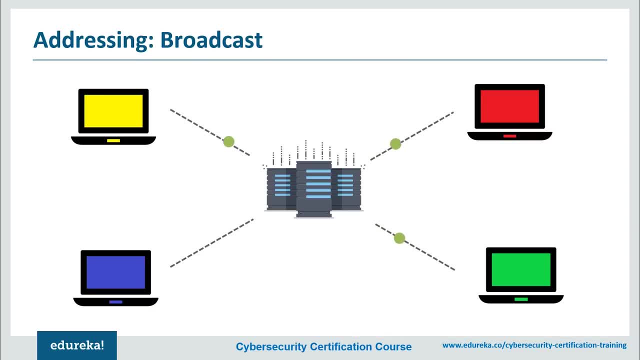 is the term used to describe communication, where a piece of information is sent from one point to all other points. in this case, There is just one sender, but the information is sent to all connected receivers. now, broadcast transmission is supported on most lands and may be used to send some messages. 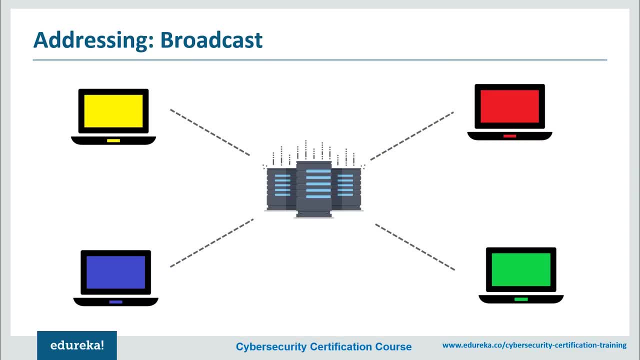 to all computers on the land. example, The address resolution protocol uses this to send an address resolution query to all computers on the land. now, network layer protocol such as ipv4 also support a form of broadcast that allows the same packet to be sent to every system in a logical network. last, 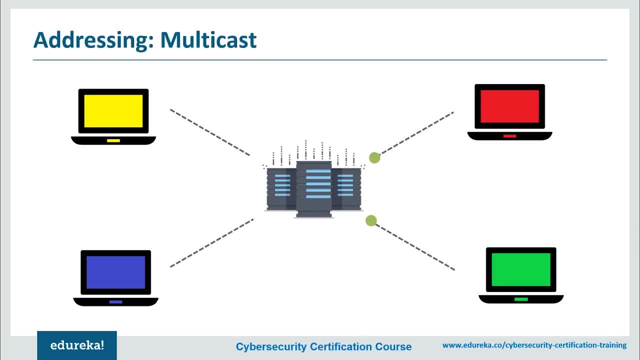 but not the least, is multicast. now, multicast is a term used to describe communication where a piece of information is sent from one or more points to a set of other points. in this case, There may be one or more senders and the information is distributed to a set of receivers. one example: 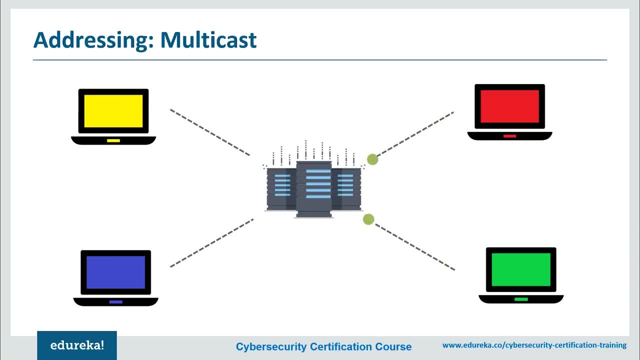 of an application which may use multicast is a video server sending out network TV channels simultaneously. delivery of high quality video to each of large numbers of delivery platforms will exhaust the capability of even a high bandwidth network with a powerful video clip server. This poses a major scalability issue. 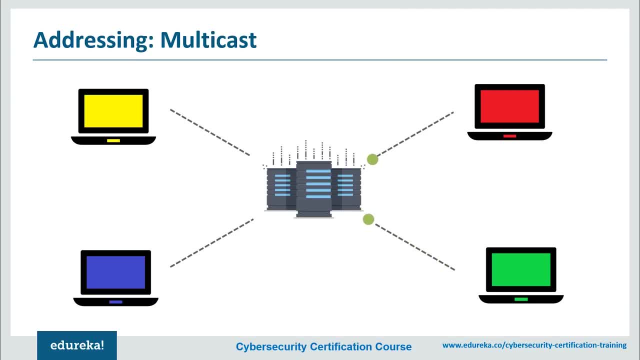 for applications which require sustained high bandwidth. One way to significantly ease scaling to larger groups of client is to employ multicast networks. Now, unlike broadcast transmission, multicast clients receive a stream of packets only if they are previously elected to do so. membership of a group is dynamic. 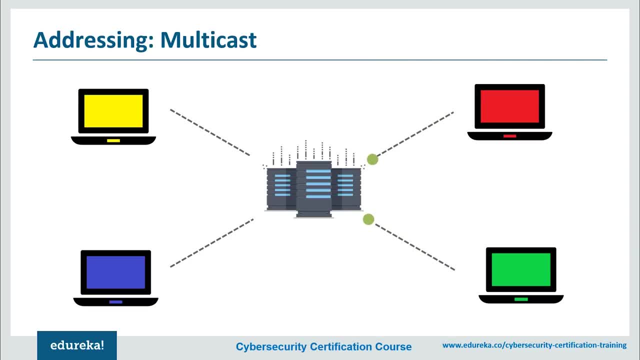 and controlled by receivers and the router in a multicast network, learned which sub networks have active clients for each multicast group, and attempts to minimize the transmission of packets across parts of the network for which there are no active clients. Okay, so let's see, We've done. 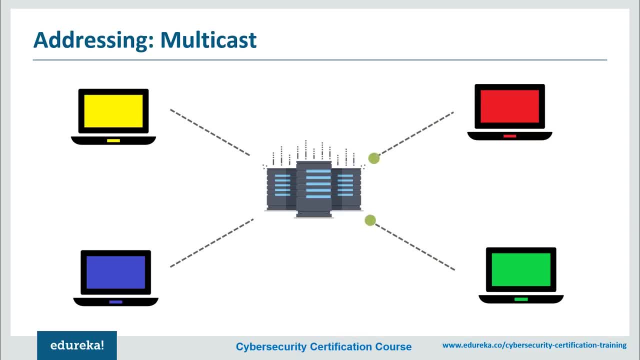 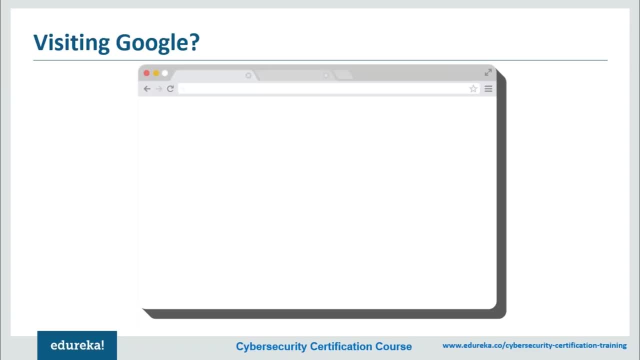 we've discussed the various types of addressing the fundamental unit of a network and the network architecture that are widely followed. Now let's see how connection is actually established when you actually make a request. So suppose you're on a browser and you type wwwgooglecom and hit enter. 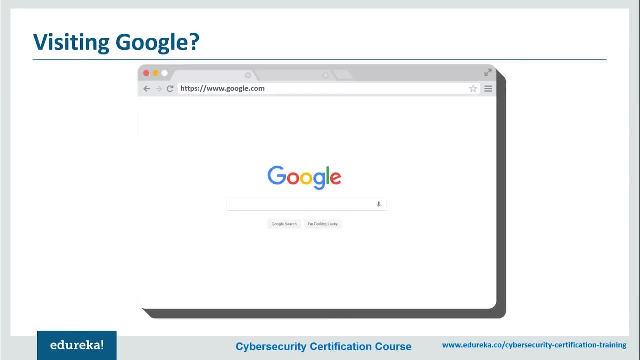 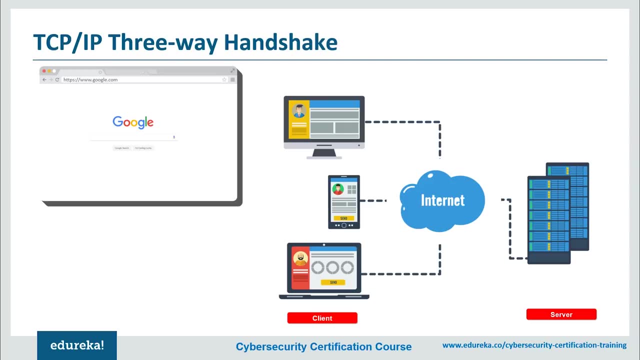 Now, when you hit enter, a series of transactions takes place. Firstly, a packet called a sin packet is sent from your computer all the way across the network to the IP address of the Google server. We'll get to IP addresses in just a bit. now, when Google server receives the sin packet, it realizes 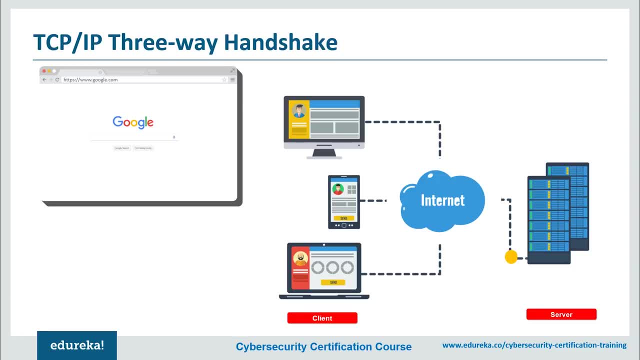 that we are trying to establish a connection with Google. So Google sends back a sin act packet which stands for acknowledgement. This is basically a way to say: hey, I acknowledge the fact that you're trying to connect to me. now This act packet is sent. 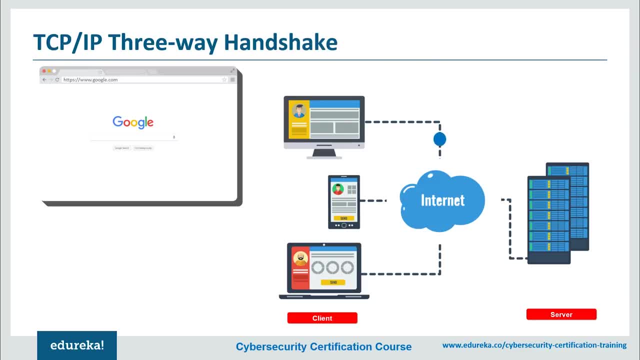 to our computer all across the network. Finally, when our client computer receives the sin act packet, it sends back another packet called the ACK packet, which basically is an acknowledgement of an acknowledgement. now, after the sin act packet is received by Google, a connection is set up between your computer and the Google server. 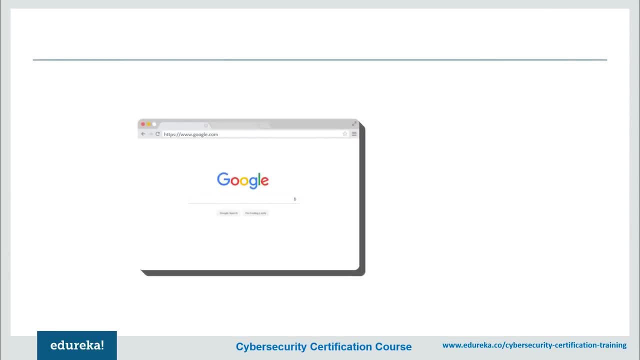 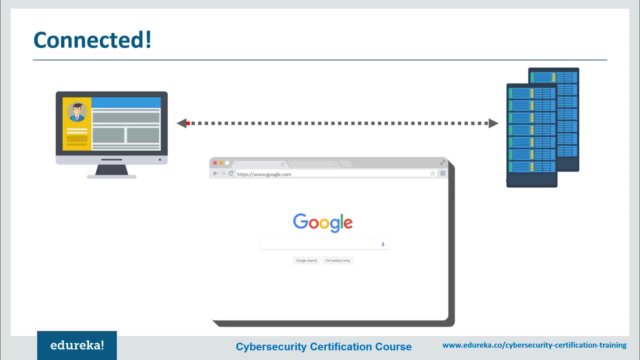 This process is the famous three-way handshake now in TCP. basically, every packet comes with an ACK packet to say, Yep, I got it, And if you don't get an ACK, you resend it. now, since this is a two-way communication, you want to make sure that your desire to connect got. 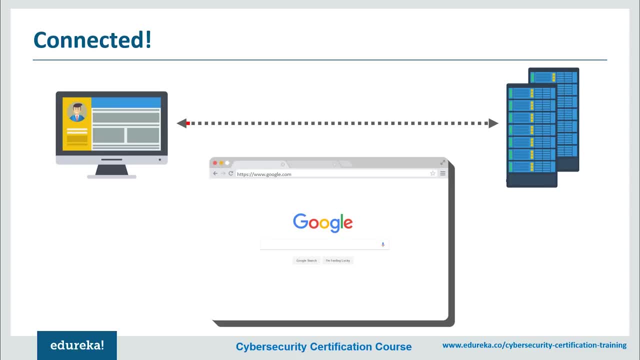 through to the receiving computer and thus they send back the sin act packet. and they want to know that whether you got their acknowledgement or not. So you send back the acknowledgement of an acknowledgement, which is basically the ACK packet. now both parties have positive confirmation that the other party has received. 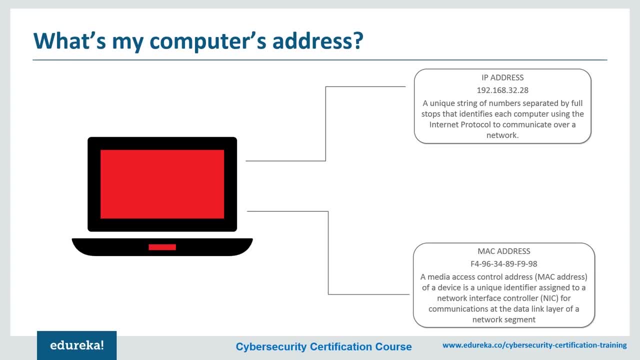 and agreed to their request to connect. now, a good question might have arised in some of your minds, that how does one know who is what on a network? Well, that is solved by the computer's address, which is basically divided into two address. one, the physical address, which is the MAC address. 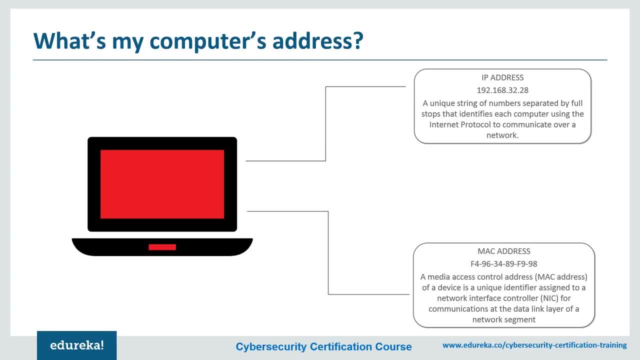 and one, the digital address, which is the IP address. and the IP address, also short for internet protocol address, is an identifying number for a piece of network hardware. having an IP address allows a device to communicate with other devices over an IP based Network like the internet. 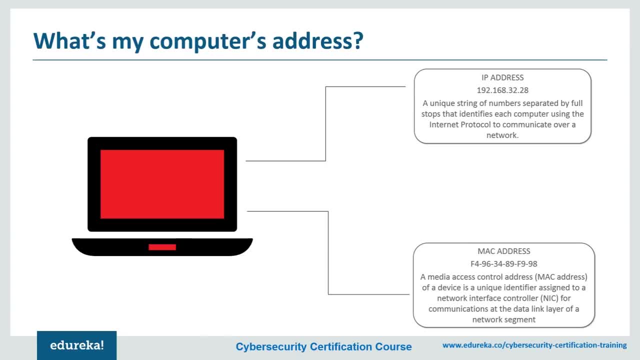 Now most IP addresses look something like four numbers that are divided by three dots. For example, 151 dot 101. dot 65 dot 121.. That's probably valid IP address. Now, if I'm going to send a packet to my friend in another country, 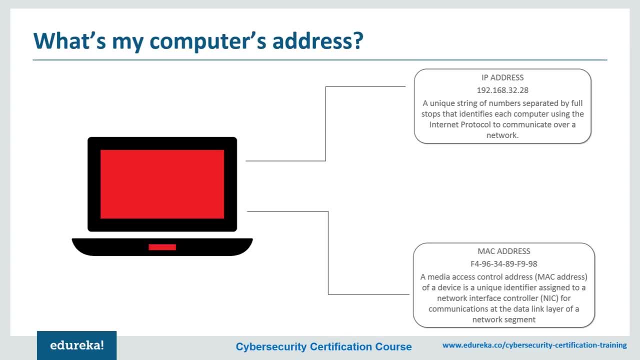 I have to know the exact destination. It's not enough just to put a package with his name on it through the mail and expect it to reach him. I must instead attach a specific address to it, which you could do by looking it up in a phone book. 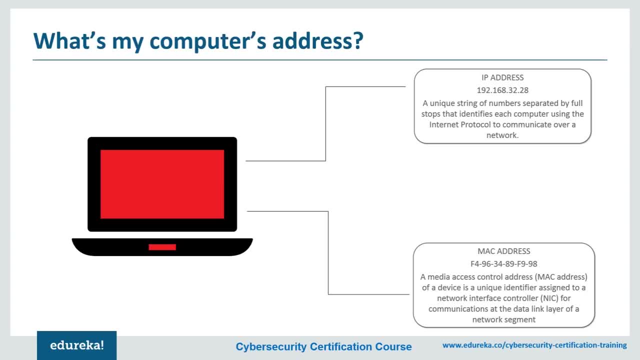 This is exactly what the IP address is. You can generally find your own IP address by typing in ipconfig on Windows system or ifconfig on a Linux based system. Now, moving on to MAC addresses. Well, in a local area Network or other networks, the MAC address is your computer's unique hardware number. 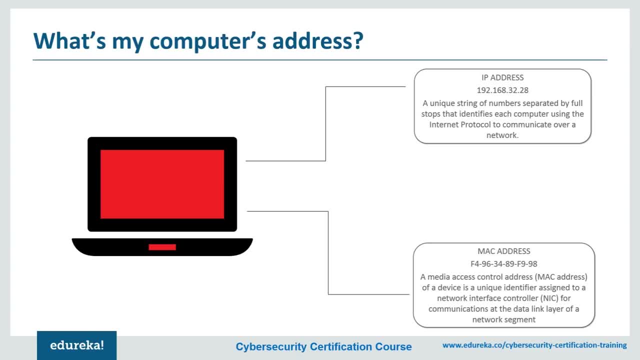 when you're connected to the internet from your computer, a correspondence table relates your IP address to your computer's physical address or MAC address. The MAC address is used by the media access control sub layer of the data link layer of telecommunication protocols. There is a different MAC sub layer. 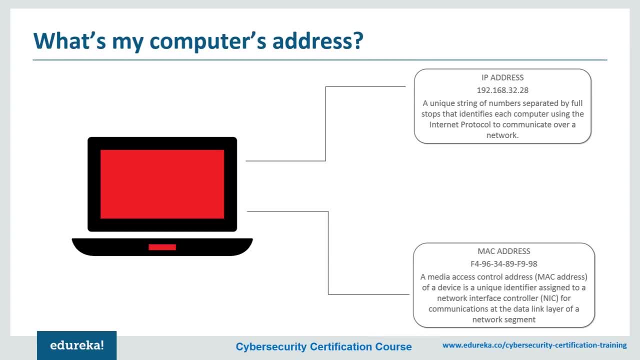 for each physical device type. The other sub layered levels in the DLC layer is the logical link control sub layer. Now, if you have access to the internet from a local area Network in your home or business, it is possible that you share an IP address with some other user. 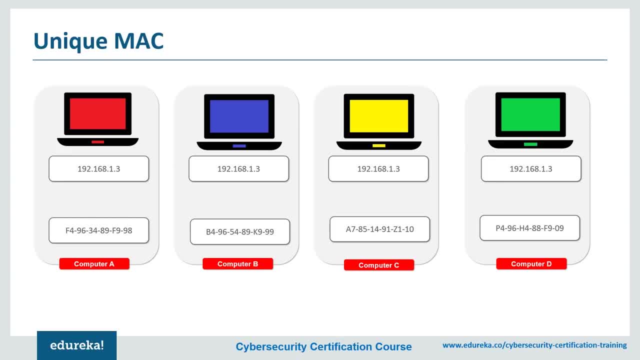 This is because, while you might use a different computer or device, you all use the same internet connection or the same access Gateway. now, in the early days of the internet, people connected to their modem directly to their computer. after all, most homes only had one computer. today, most homes contain several devices. 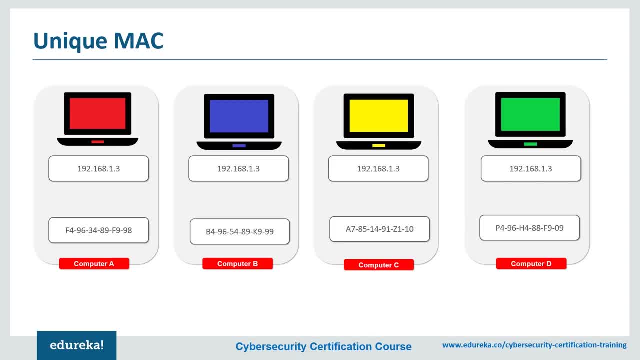 that connect to the internet. Therefore, it is far more common to connect a DSL or cable modem to a router that can be accessed by multiple devices. Now some modems even include a built-in wireless router. Now your router gives each connected device a unique. 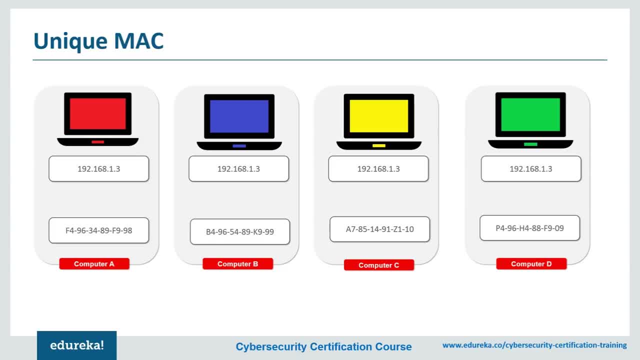 internal IP address that distinguishes differently on different local networks. This address are automatically distributed by the router using a protocol called DCHP. Typically, IP addresses of local devices might be 10.1.1 or 10.0.1.3, and some routers may also use the IP address. 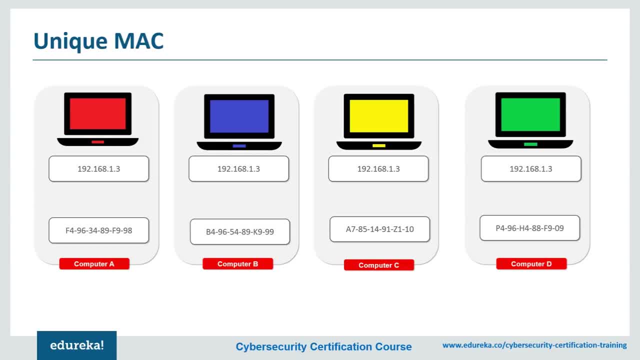 that use the whole 192.168.xx format, But this is not true for MAC addresses. Every device on this planet has a unique MAC address. MAC, or media access control address, is a globally unique identifier assigned to a network device, and therefore it is often referred to as a hardware or physical address. 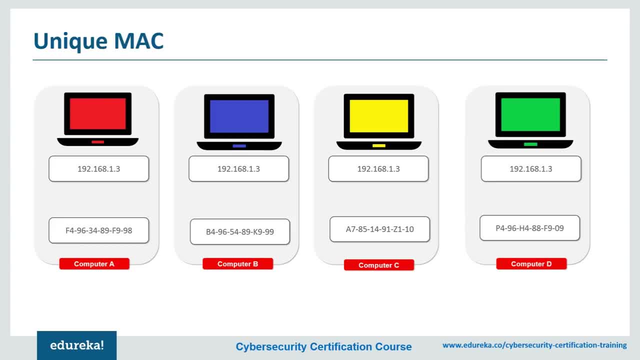 MAC addresses are of six bytes. The first three bytes are ID numbers of the manufacturer, which is assigned by an internet standards body, and the second three bytes are serial numbers assigned by the manufacturer itself. Okay, so that was about MAC addresses and IP addresses. 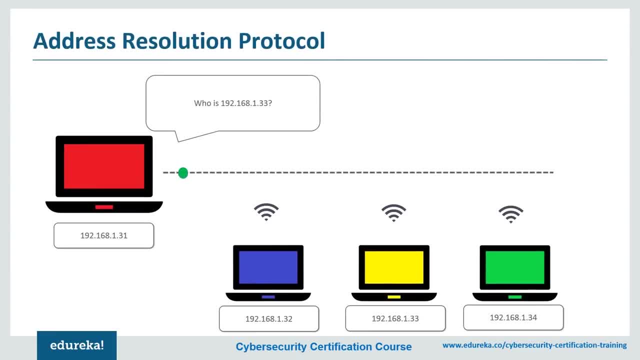 Now what happens when you're actually trying to connect to some other computer on a local area network? So when you're on a local area network, a certain protocol- ARP, which stands for address resolution protocol- is used to communicate with other devices on the network. The term address resolution refers to the process of finding 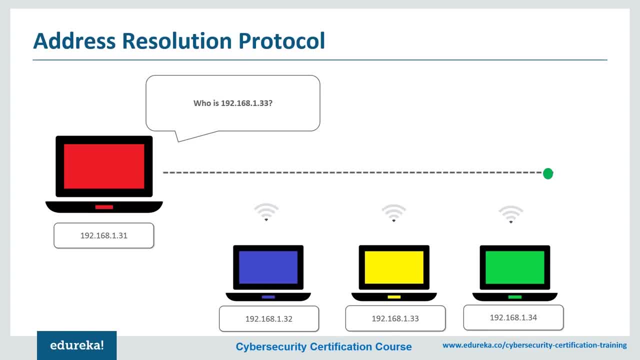 an address of a computer in a network. Now the address is resolved using a protocol in which a piece of information is sent by a client process executing on the local computer to a server process executing on a remote computer. The information received by the server allows the server. 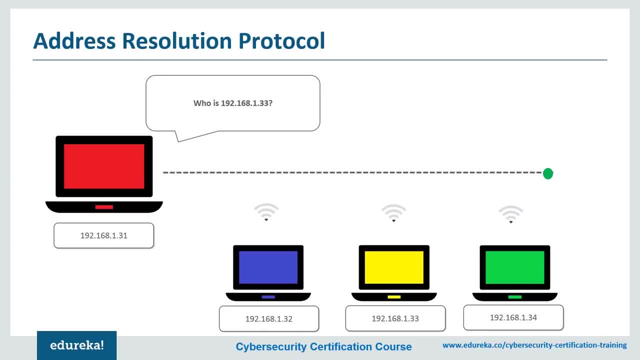 to uniquely identify the network system for which the address was required and therefore provide the required data Address. the address resolution procedure is completed when the client receives a response from the server containing the required address. Now, if you realized, ARP isn't really using a three-way. 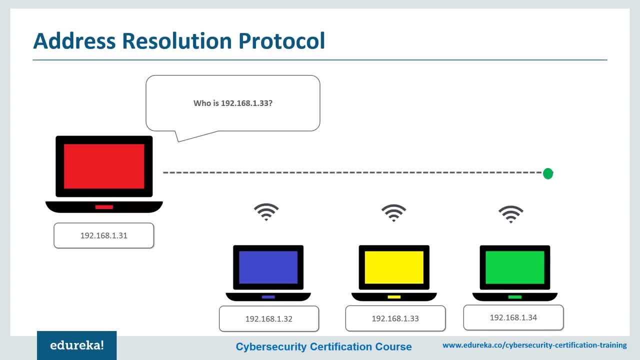 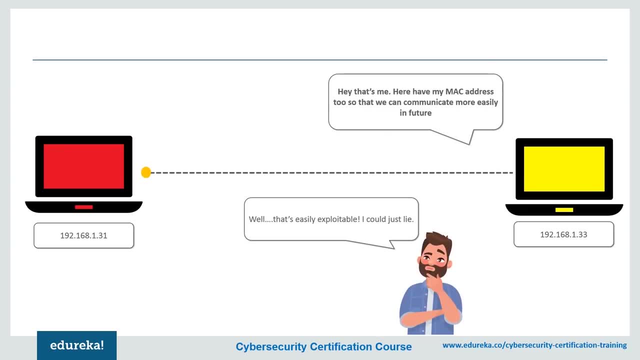 handshake mechanism or any authentication, So this can be very easily exploited. All you have to do is live and someone sends an ARP request. Now you could lie to a computer that you are the router and you could lie to the router that you are the victim computer. 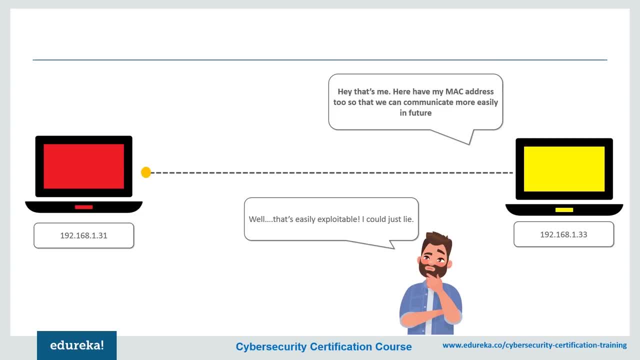 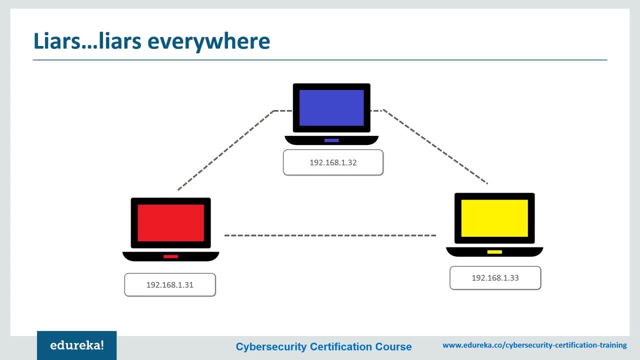 This is what we call ARP spoofing, and an attack like this is called a man-in-the-middle attack. and MITM attack happens when a communication between two systems is intercepted by an outside entity. This can happen in any form of online communication, such as email, social media, web surfing, etc. 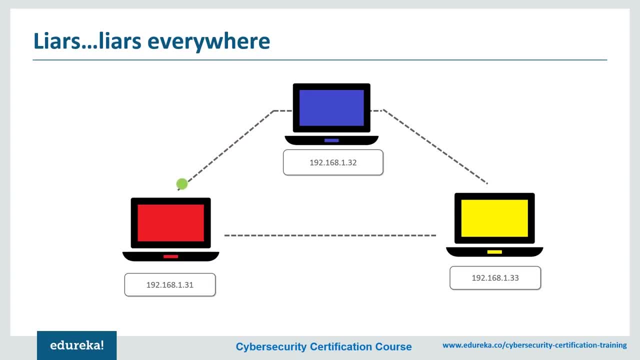 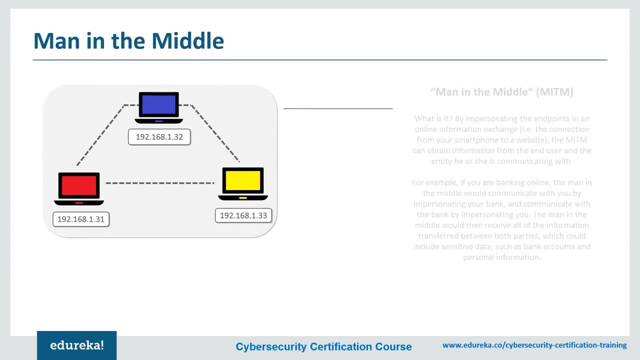 Not only are they trying to eavesdrop on your private conversation, They can also target all the information inside your device. but taking away all the technicalities, the concept of an MITM attack can be described in a simple scenario. Now imagine being brought back to the days. 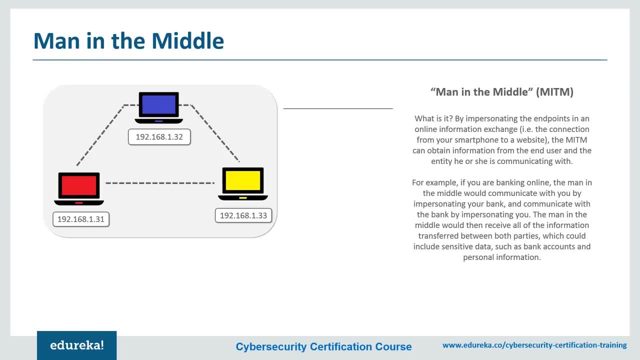 when old snail mail was being used. Jerry writes a letter to Jackie expressing his love for her after years of hiding his feelings. He sends the letter to the post office and it is picked up by a noisy mailman. He opened it and just for the hell of it. 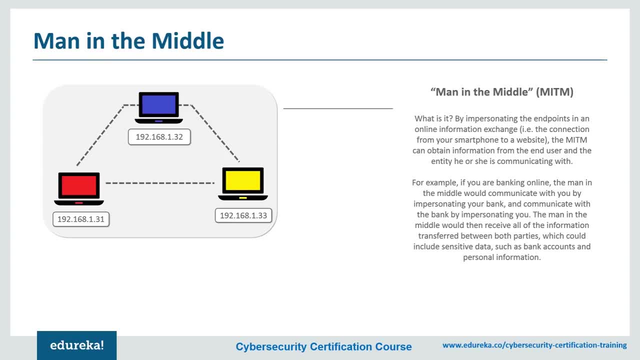 he decided to rewrite the letter before delivering the mail to Jackie. This results in Jackie hating Jerry for the rest of her life, after Jerry called her a fat cow on their letter. The moral of the story is: the mailman is a jerk and so are all the hackers that do the same. 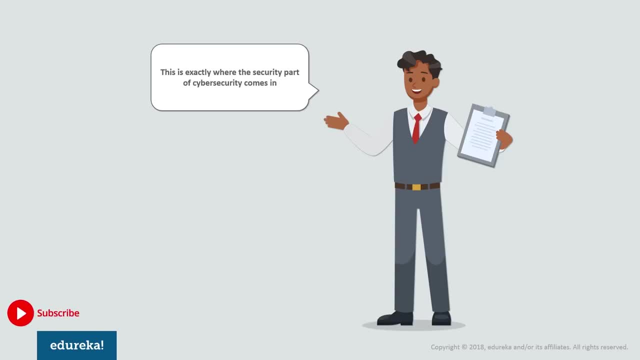 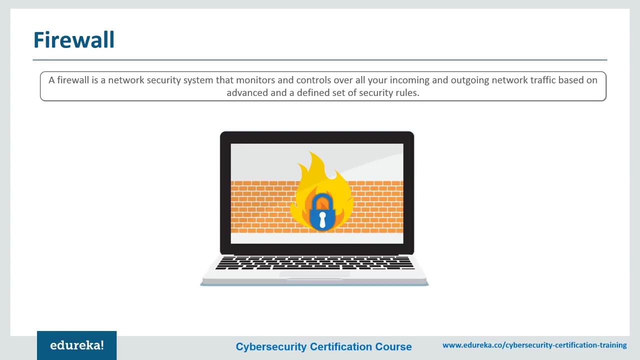 This is exactly where the security aspect of network security comes into play, to protect our data from unauthorized access, unauthorized modification and unauthorized deletion. and the most common type of security measure that every computer uses is a firewall. A firewall is a software or firmware that enforces 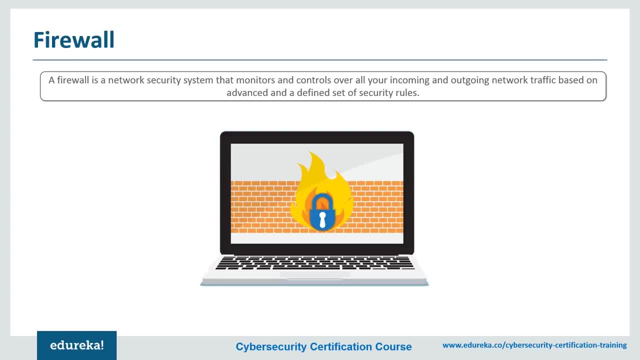 a set of rules about what data packet will be allowed to enter or leave a network. firewalls are incorporated into a wide variety of network devices to filter traffic and lower the risk that malicious packets traveling over the public internet can impact the security of a private network. now firewalls, while they come pre-installed, 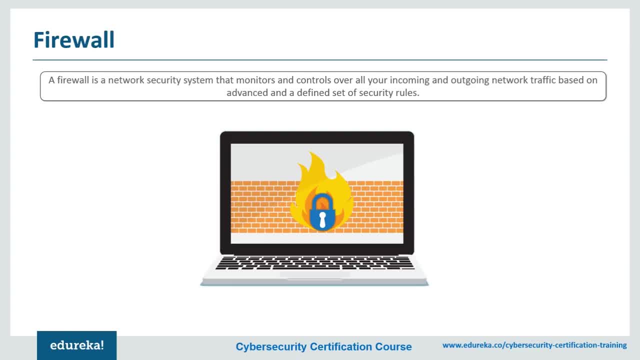 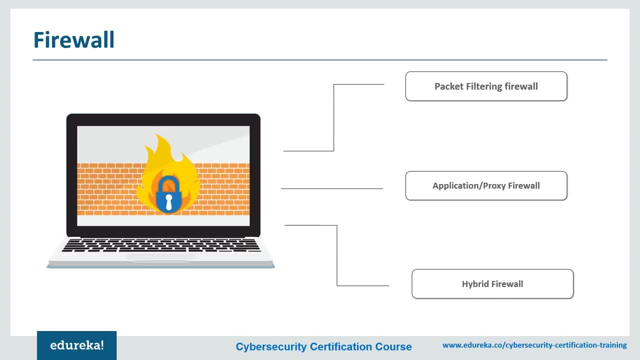 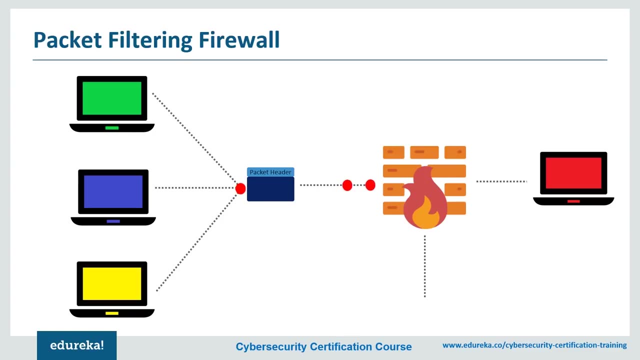 can also be purchased as standalone software applications. Now, generally speaking, There are three types of firewalls: packet filtering firewalls, application or proxy firewalls and hybrid firewalls. Let's look at packet filtering firewalls first. now, packet filtering firewall: just check the packet header of packets. 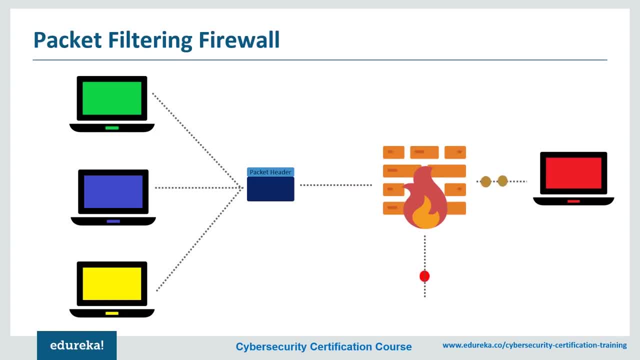 that are being sent to your computer. They analyze the packets according to rules written in a file called ACL, which stands for access control list. packet filtering firewalls are already installed in our router and provide the cheapest form of security, but it is underwhelming as a payload is not checked. 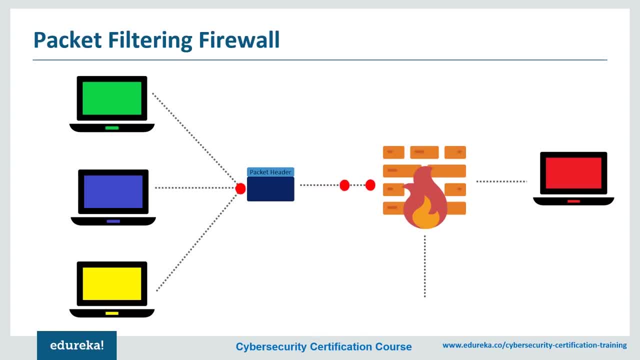 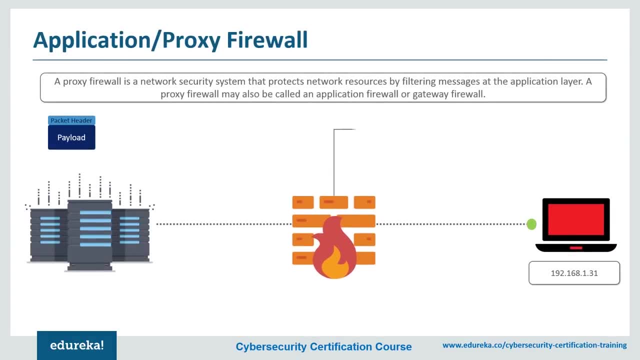 So basically it checks the packet header but not the payload. So it's not a very good type of firewall, but it always comes pre-installed in a computer. Next up is application firewalls, which are completely different from packet filtering firewalls. 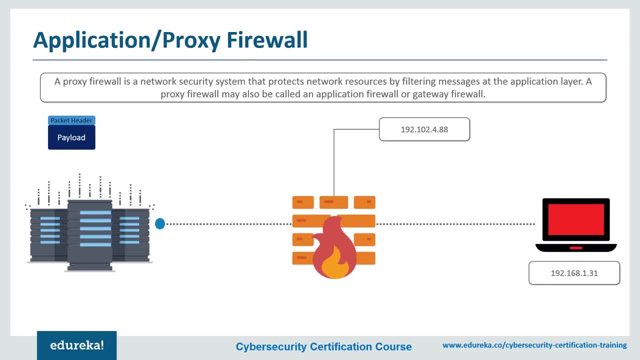 They check both the payload and the packet header. and, above that, proxy firewalls have their own IP address. So when you access the internet through the proxy firewall, you're actually hiding yourself from malicious users by masking your IP with your firewalls IP. This is the basic principles on how proxy servers 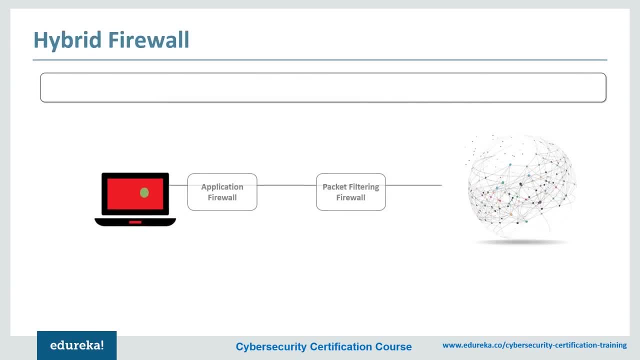 and proxy firewalls work. last but not the least is a hybrid firewall, which is the combination of application firewall and a packet filtering firewall. They provide much higher security, but it should be noted that they must be applied in series when they're applied in parallel. 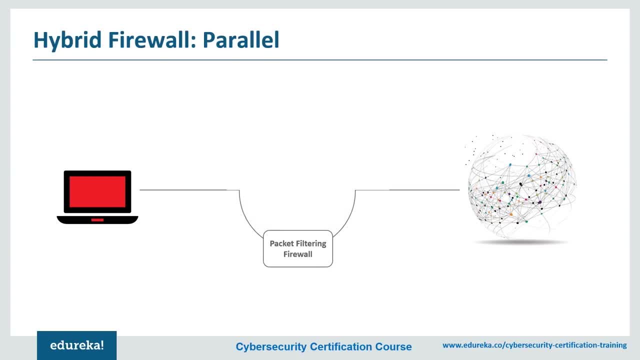 The security is brought down to the level of a packet filtering firewall, and the networks act like the proxy. firewall doesn't exist at all. Now, that was all about firewalls, but in all honesty, it is comparatively much easier to break a firewall than modern encryption systems. 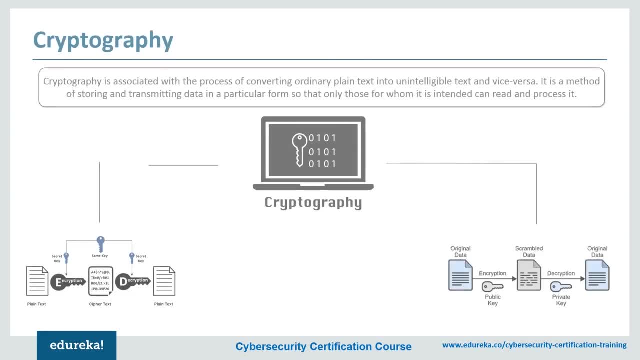 which are used to protect data. So when talking about encryption, we are talking about cryptography. Now cryptography comes in two flavors, namely symmetric cryptography and public key cryptography. So first let's discuss symmetric key cryptography. Now an encryption system in which the sender 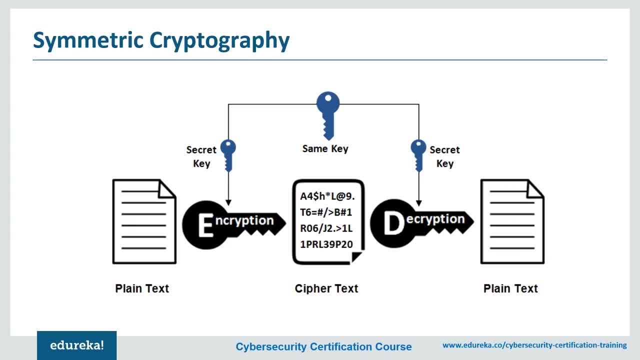 and receiver of a message share a single common key that is used to encrypt and decrypt a message is called symmetric key cryptography. Now, this contrasts with public key cryptography, which utilizes two keys: a public key to encrypt a message and a private key to decrypt them. 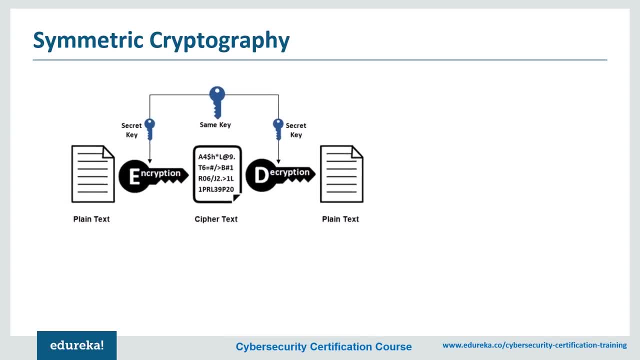 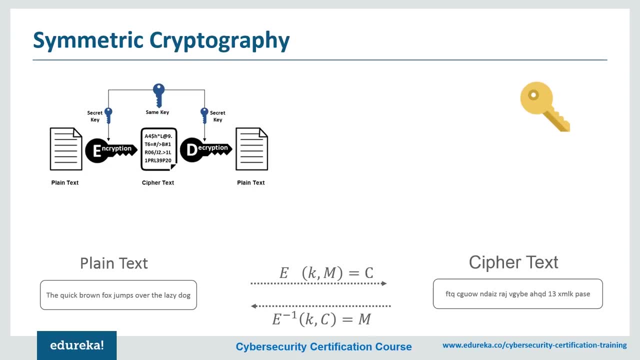 Secret key systems are simpler and faster, but their main drawback is that two parties must somehow exchange the keys in a secure way. Public key encryption avoids this problem, because the public key can be distributed in a non-secure way and the private key is never transmitted. 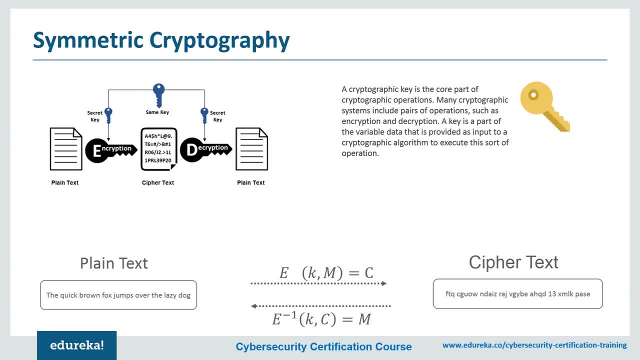 Now, symmetric key cryptography is sometimes also called secret key cryptography, because the security of this whole encryption algorithm depends on how secret you can keep your key. Now, cryptography key is a core part of a cryptographic operation. Many cryptographic systems include a pair of operations, such as encryption and decryption. 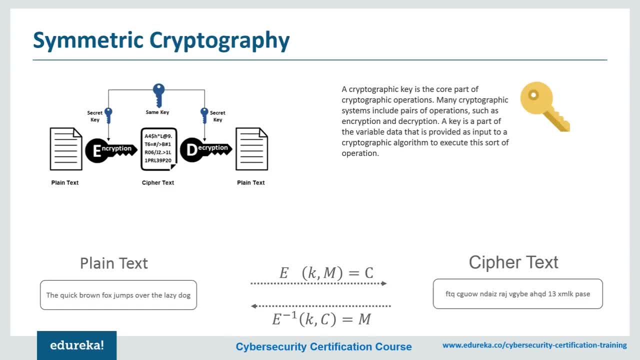 and a key is a part of the variable data that is provided as an input to cryptographic algorithms to execute the sort of operation. Now, in a normal symmetric key cryptography, you'd probably have a plain text. Suppose the plain text, which is: the quick brown fox jumps over the lazy dog. 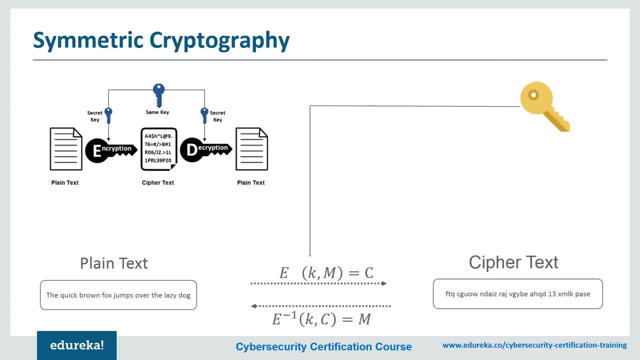 which is put into an encryption algorithm which contains the key and the message, and you get a ciphertext. Now the ciphertext is then also put into a decryption algorithm which uses the same key, and then you get the plain text that produced the ciphertext. This is how simple symmetric key cryptography works. 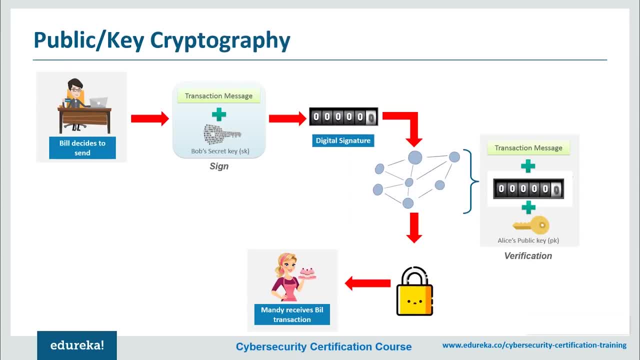 Now, in public key encryption systems, any person can encrypt a message using a receiver's public key. That encrypted message can only be decrypted with the receiver's private key. So to be practical, the generation of a public and private key pair must be computationally economical. 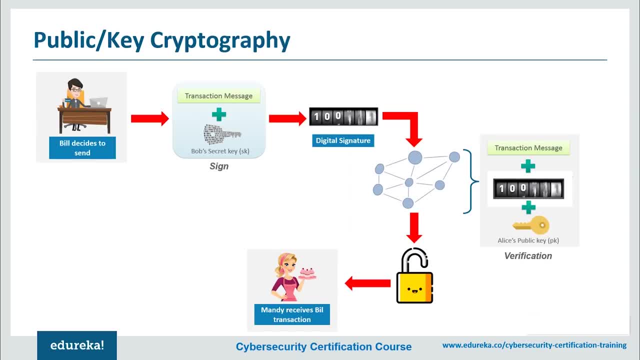 Now, the strength of a public key cryptography cryptographic system relies on computational effort or the work factor in cryptography that is required to find the private key from it pairs public key. So effectively, security only requires keeping the private key private and the public key can be distributed. 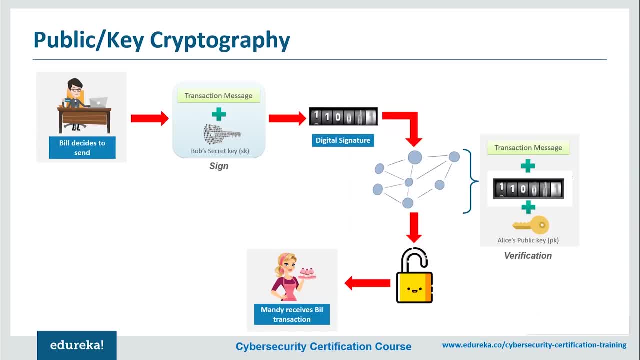 without compromising security. Public key cryptography systems often rely on cryptographic algorithms based on mathematical problems, particularly those inherent in certain integer factorization, discrete logarithms and elliptic curve relationships. Public key algorithms, unlike symmetric key algorithms, do not require a secure channel for initial exchange. 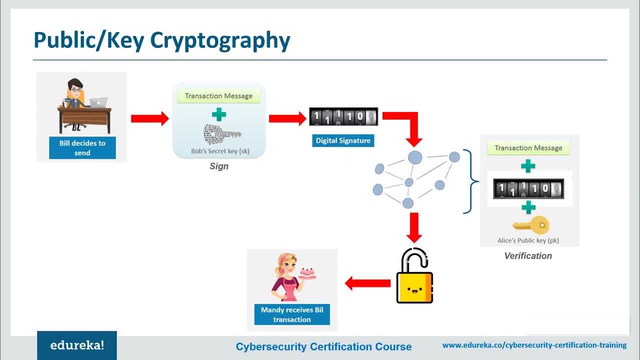 of one or more secret keys between the two parties. So, because of the computational complexity of asymmetric encryption, it is usually used only for small blocks of data, Typically the transfer of a symmetric key encryption system. This symmetric key is then used to encrypt the rest. 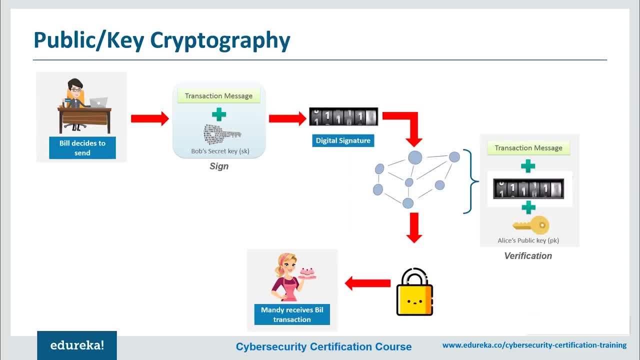 of the potentially long message sequence and the symmetric key. encryption and decryption is based on a simpler algorithm that works much faster. So, because of the computational complexity of asymmetric encryption, it is usually used only for small blocks of data, Typically the transfer of a symmetric encryption key. example: a session key. 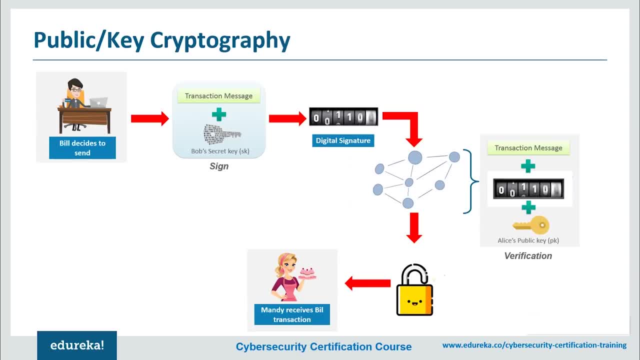 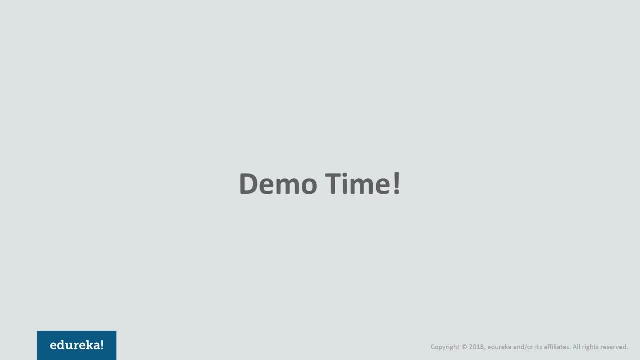 Now this symmetric key is then used to encrypt the rest of the potentially long message sequence, and the symmetric encryption and decryption is based on simpler algorithms. that is much faster, Okay, So now it's time for an interesting demo on why you actually should really be aware. 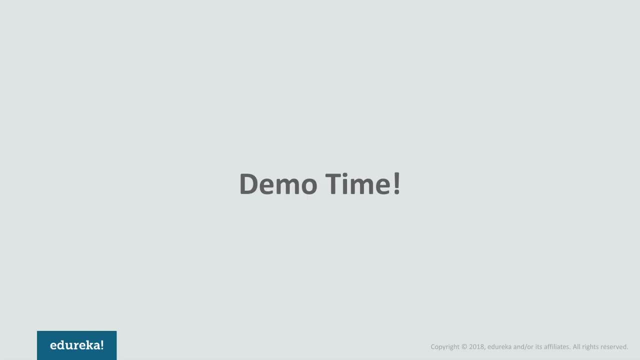 of cyber security. So for this demonstration, I'm going to be showing you guys a man in the middle attack. So for the man in the middle attack, as we earlier discussed, we are going to need to ARP spoof ourselves to another computer and ARP spoof ourselves to the router too. 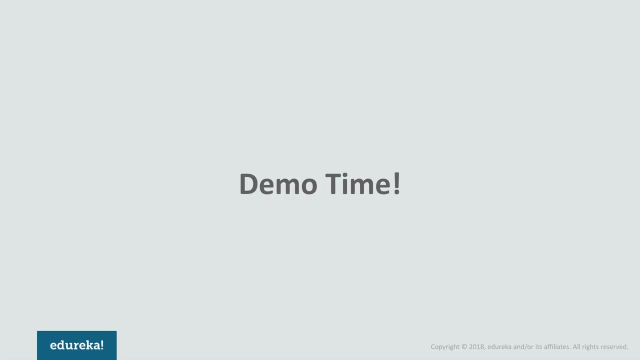 So that means we are going to fool the computer that we are the router and then we're going to fool the router that we are the computer. So for this demo I'm going to be using two machines. one is going to be running Linux and on the Linux based machine 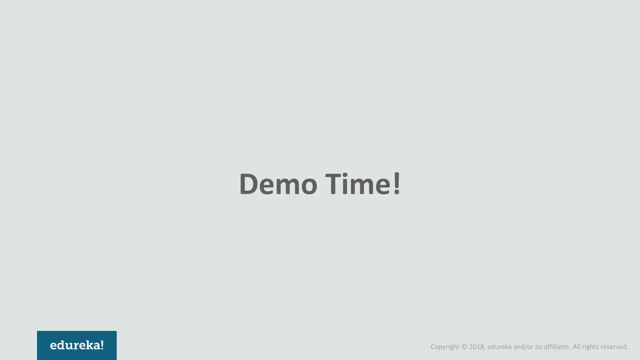 I'm going to be performing the attack and for the victim I've chosen it to be my own machine. and for the results, you guys will see how I'm going to sniff out all the images that is being served on the victim machine. Okay, 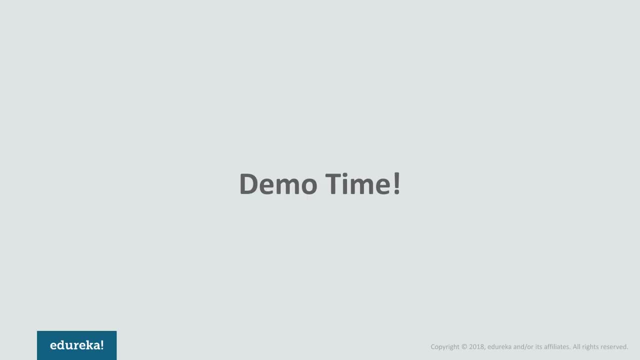 So for this demonstration, we are going to be using framework called WebSplit. Now, WebSplit is an open-source framework and it's easily available on Linux, and it can help simulate man-in-the-middle attacks, just for educational purposes. So let's get started. 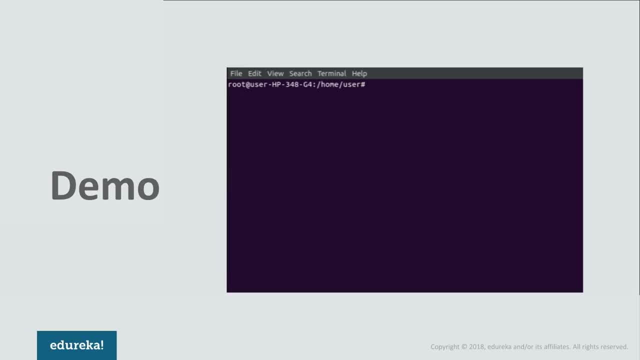 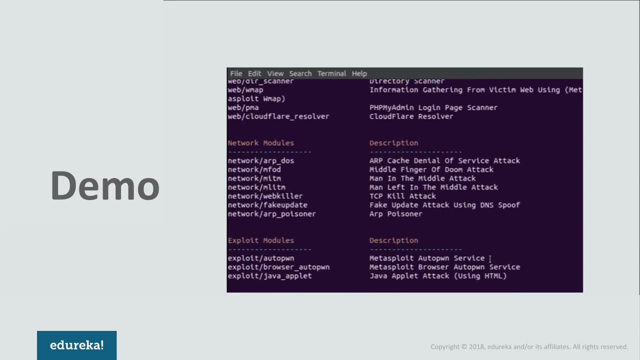 So first of all, we are going to start up WebSplit by typing in the command WebSplit. So once you go into WebSplit you go show modules. So, as you guys can see, we have so many modules available out here and these are all the types of attacks. 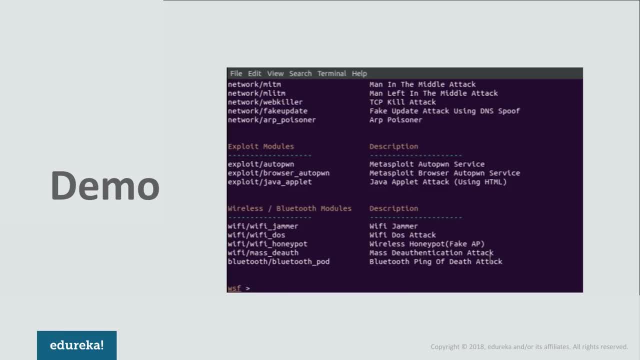 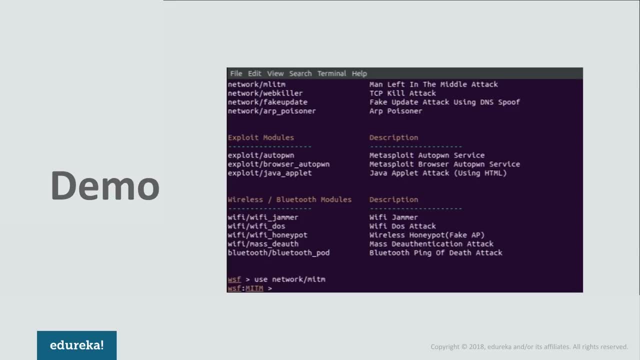 that you could possibly simulate with this framework. So we're going to choose the man-in-the-middle attack. So that is, we're going to use network slash MITM. So now you're going to see all the options that we are having. So, as you guys can see out here, 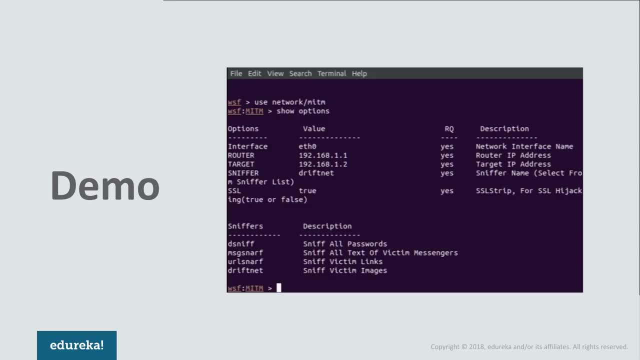 the WebSplit framework gives us numerous amounts of options to set up. First we can set the interface that we're going to attack on, and then we can also set the router that we're going to attack through. then we can set these target IP address and we can also set from a number of different sniffers. 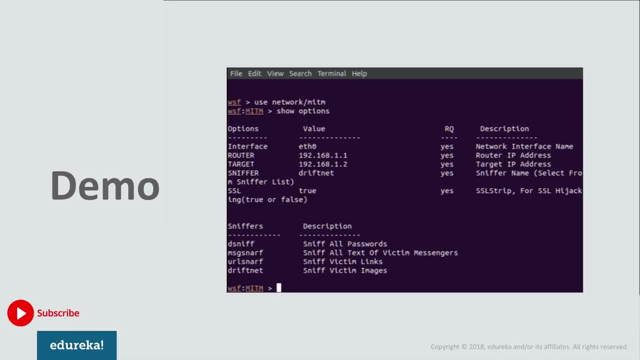 For example, we can use drift net for sniffing out victim images. We can use URL snarf for sniffing out victim links. Then we can use DSNF for sniffing out all sorts of passwords. Also, we are going to use SSL strip. 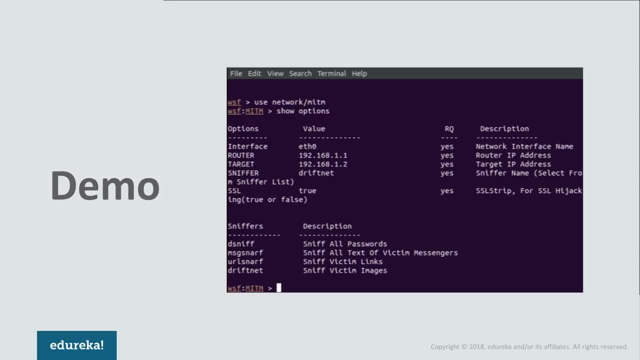 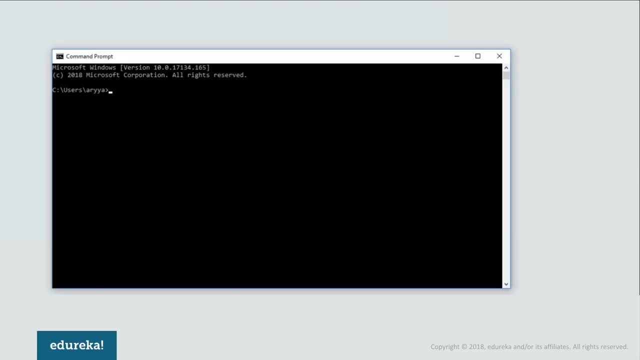 for actually stripping down SSL protocol, so that you're not actually visiting a secure site. So firstly, we need the IP address of our victim site on this computer. So I'm going to go on my computer and check out my password. So IP config. 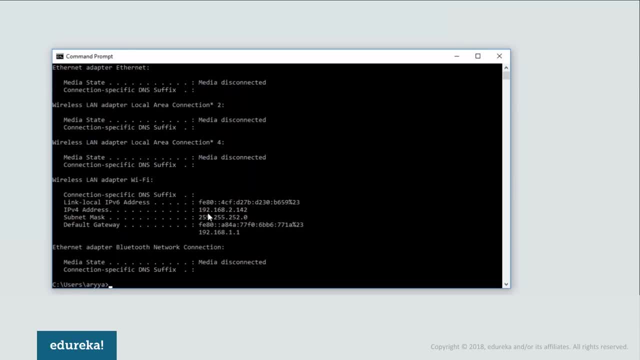 So, as you guys can see, my password out here is 192.168.2.142 and my default Gateway is 192.168.1.1.. So that means my computer- This is .2.142- is connecting to the router, which is then connecting to the rest of the internet. 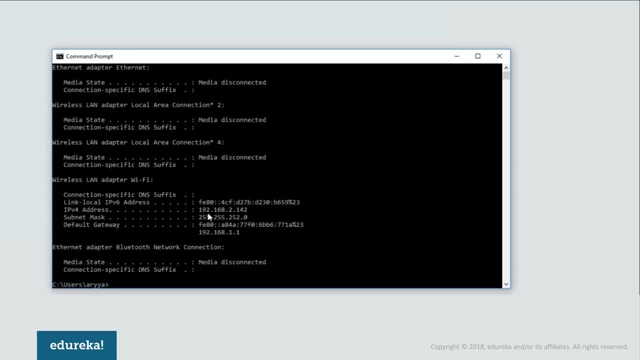 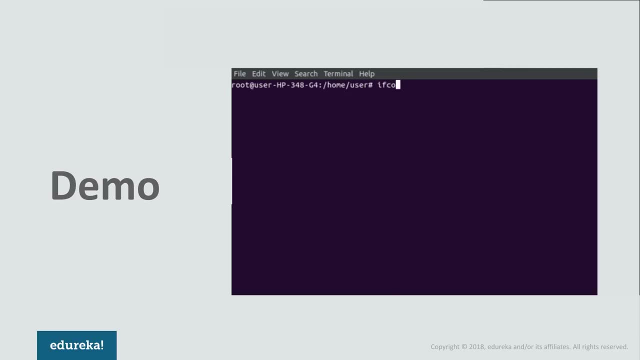 through 192.168.1.1.. So to check out my attacking computers IP address, I'm going to go to my computer and go ifconfig and we see that we're running on the interface wlp2so You can also check that by going route hyphen n. 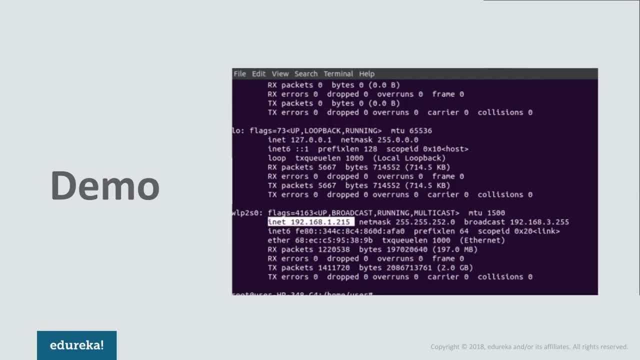 and this will show you the Gateway, that it's 192.168.1.1 out here, as you guys can see, and our IP address is out here 192.168.1.215.. So this is our attacking IP address. So, moving on to web split now. 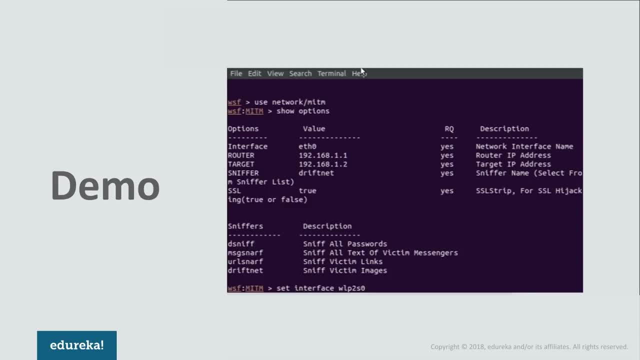 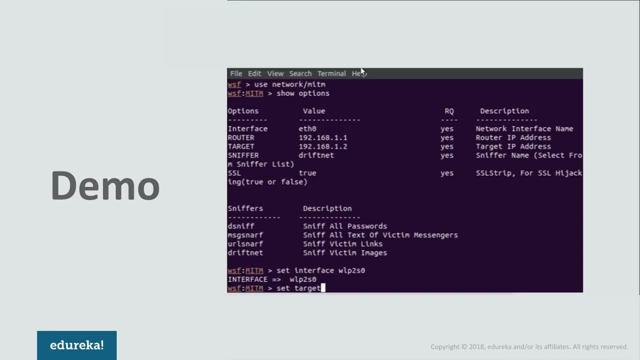 Okay, So first we need to set our interface, So we go set interface. So that sets our interface. Then we need to set the target, as the router IP address is already correct. So our target is going to be 192.168.2.142. 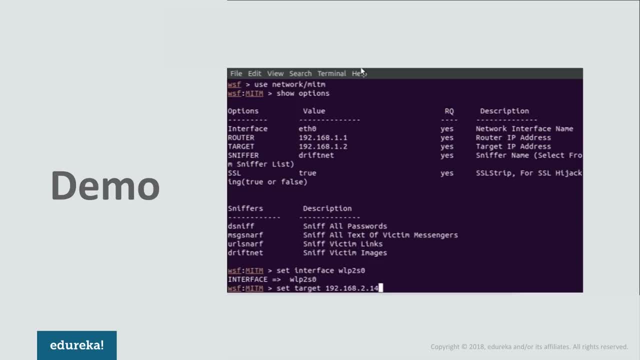 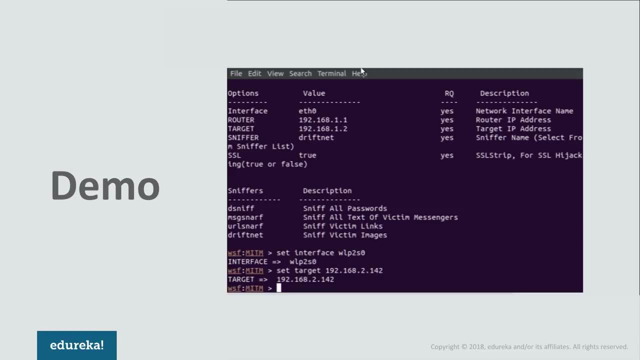 192.168.2.142, and we're going to use the driftnet sniffer for sniffing out all the victim images and SSL is true, So let's just check we've got everything correctly. Show options. So yes, our interface has been set.